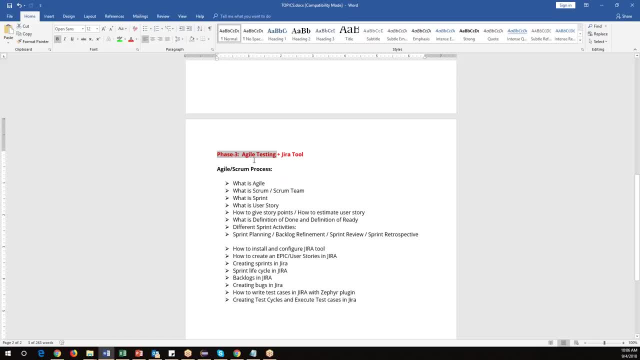 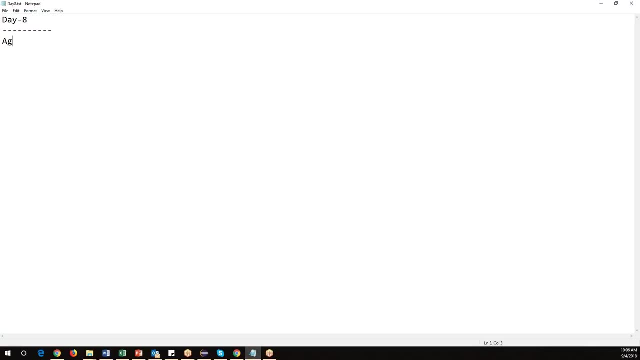 completely by taking a small project, Okay, And we can also automate this complete agile process by using Jira tool. So we will also going to discuss about Jira tool, how we can automate all these activities in Jira tool. Fine, So now today let us talk about agile process, So how the software development will be happening in the agile process. This is the latest model. currently, the market- 90% of the markets- are following. 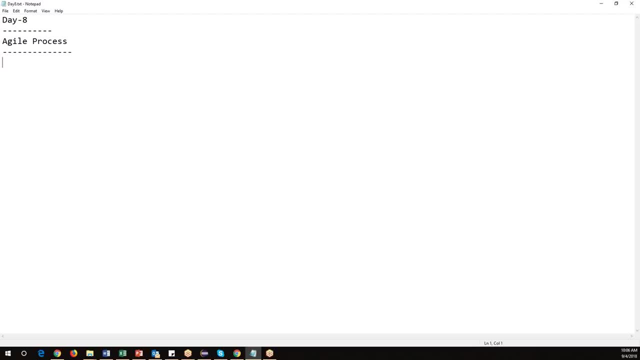 Companies are following agile process. Now let us see what is agile, how the process will be and what are the different new terminologies. So so far we are, we have used like requirement and test case and different terminologies we have used, And in agile perspective we have a different kind of terms. Okay, First we need to understand them. So now let us start with the agile process. 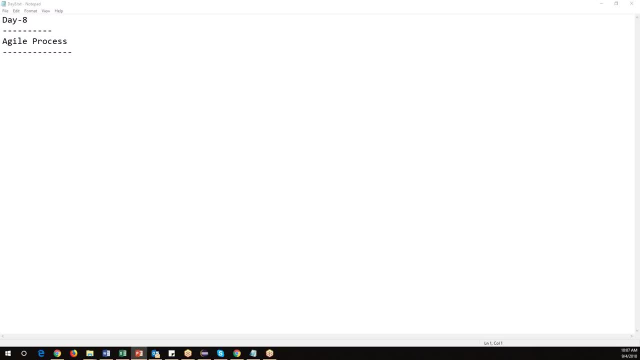 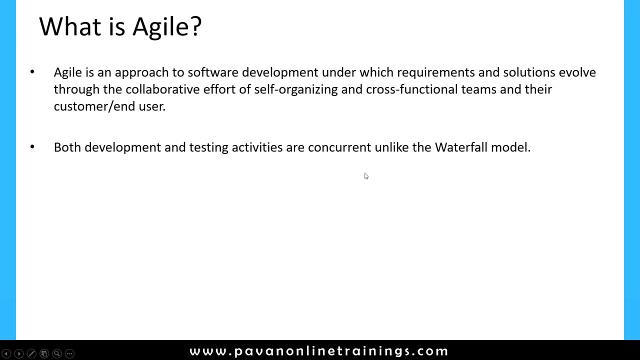 Okay, So now, what is agile process? So agile is an approach to software development under which requirements and solutions evolve through the collaborative effort of self organizing and cross functional teams and their customer and user. So, basically, agile process is talk about the collaboration. So there are a few important points which we need to remember. 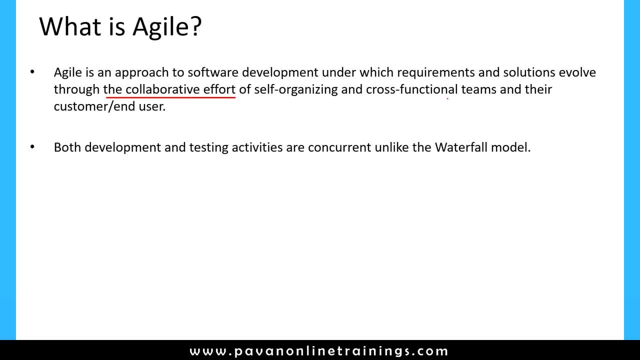 One is a collaborative effort, Okay, And requirements and solutions and cross functional teams. These are the important terms we need to understand. So agile is nothing, but it's a kind of a software development process, Just like a. previously we have waterfall model and prototype model and so on, Right And similarly we also have the agile process model. So this is also for developing a software. But what is the specialty in agile process is here's developers. 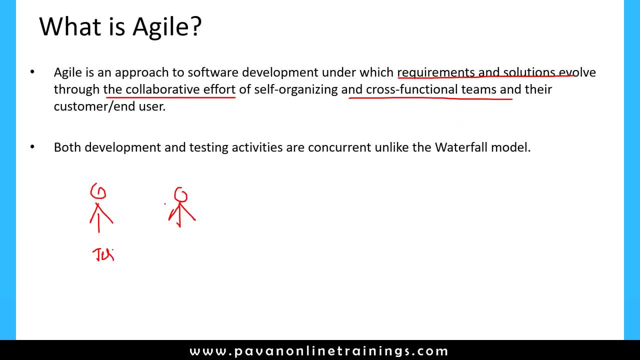 And also testers. testers and also developers will work together as a one team. Okay, That is a specialty here And this team is called as an agile team. Agile team- And one more important thing is here there is no separate teams like so all combined together we call as an agile team. So agile team is it a collection of multiple people, like testers will be there, developers, product managers and everybody will be part of this. 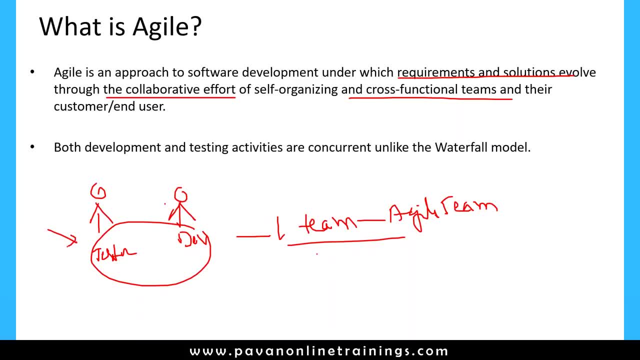 So we're talking about all kinds of roles that people participate in. If an agent does the tasks firsthand, it's independent of the engineering team, So it's coming out of the software. We don't need them anymore. They grab a main character or a student to work that matters. They into that, using these tasks firsthand. We do them if they need to do a set pre- contract or after establishment of project. 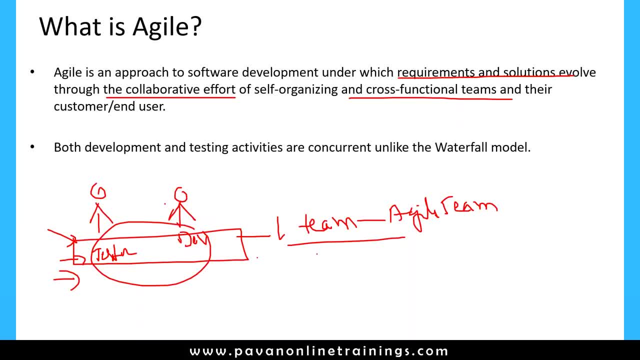 And here the role is not important, So the task, what they are performing, is very important. So here we don't have any specific alternation. So they like a: no seniors and juniors. like this, Everybody will fall under a same. So hattenigh hat receive trour also enkay. 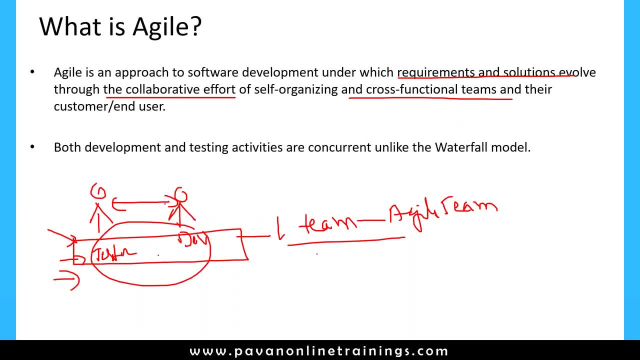 Same category, So actually a process. aze, It is not like that. So testers and developers will go both parallel, So developer do their tasks and parallelly the tester is also will perform the task, and all together everybody comes under one team. that's called agile team. 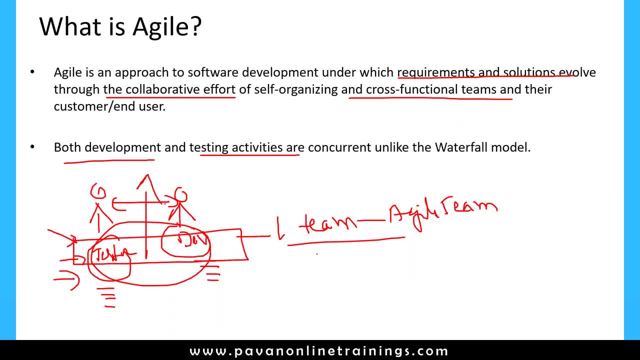 So both the development and testing activities are concurrent, unlike the waterfall model. So in waterfall model, what we have to do first we need to do analysis and the design, testing, coding, and then testing will happen right, But this is a step-by-step process. 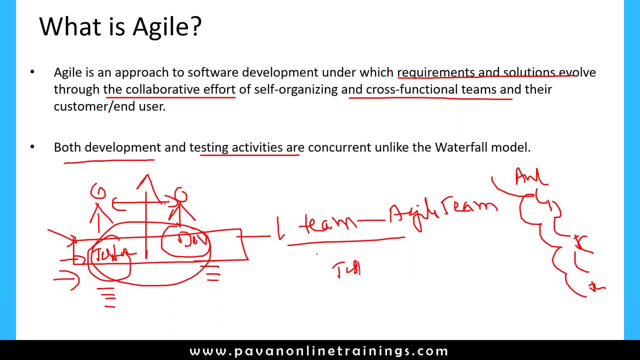 but in agile it is not the step-by-step process, So testing activities as well as development will go both parallel. okay, And here there is a lot of collaboration is required. So there is a lot of communication is required, okay. And one more advantage is we can just 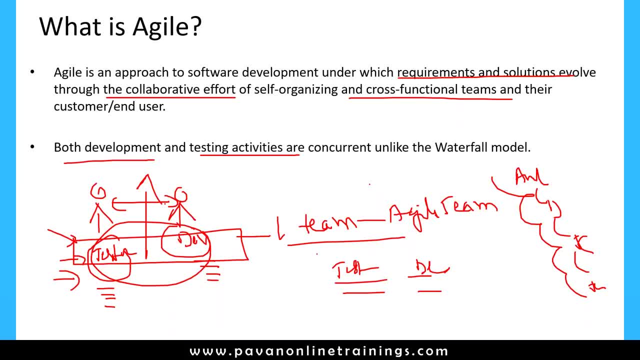 get the customer requirements and whenever the customer have changed the requirements we can just easily accommodate those requirements in this part of software development process. But in other models, like waterfall model, suppose after one month or two months the customer came and change their requirements. 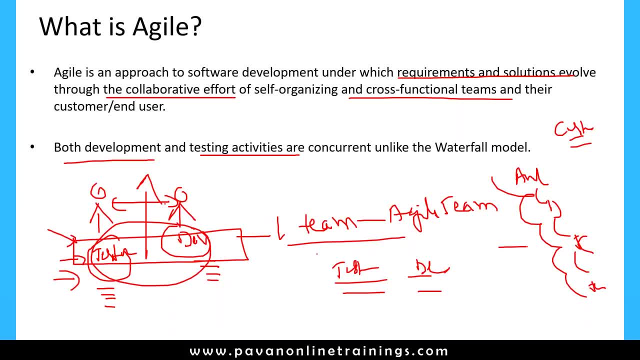 or ask to implement some new requirements, And by that time we are in the middle of software development process. So this time we can. it is little bit difficult to accommodate all the requirements or changing the requirements right So, but in agile process we can easily accommodate. 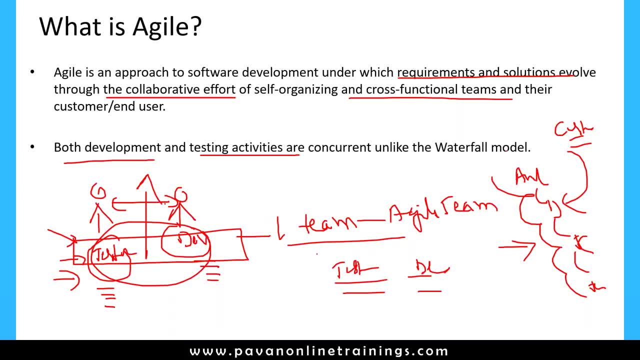 all the requirements. Whenever the changes or new requirements is added, we can easily accommodate into our development process. So that is all about agile. So agile is a software development process model where the development and as well as testing activities it will go parallelly and collaboratively. 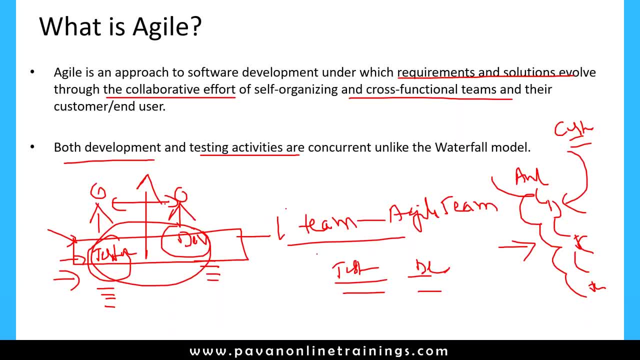 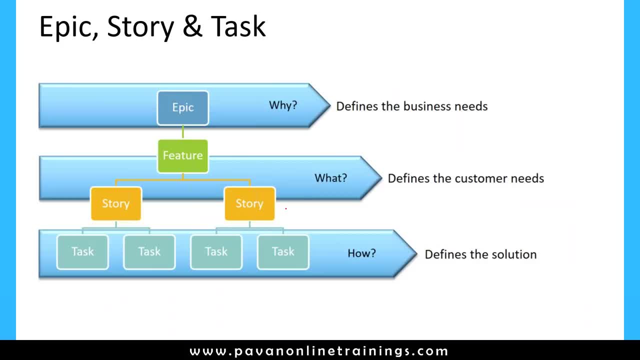 Now let us see what are the new terminologies we have to use in agile process. In agile process, before going to discuss this model, we need to understand few terminologies, And here we use very common terminologies called as epic, story and task. 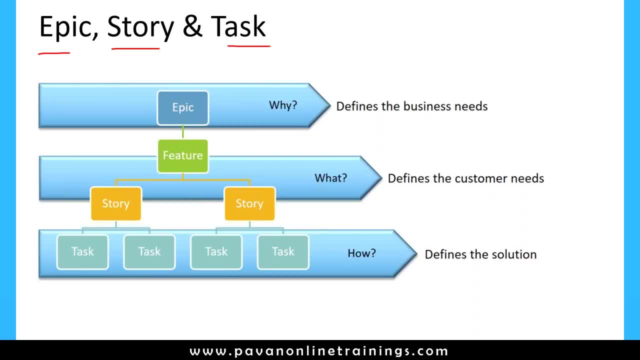 So first we need to understand this terminology. What is epic? What is story? What is task? In normal previous processes we have understood functional requirement document right. So what is functional requirement? document which contains the requirements which are specified by the customer. 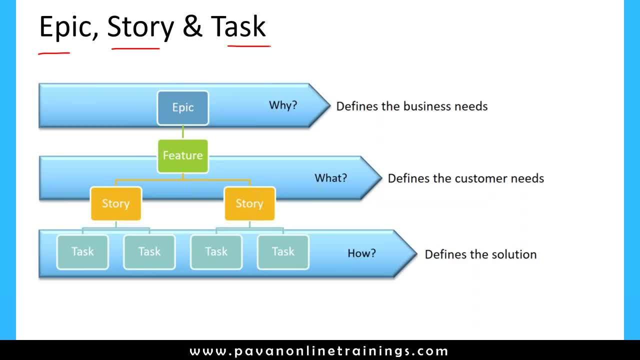 So by reading the functional requirements specification we have understood the functionality of application. But in agile process the documentation is very less. We don't have much documentation because agile is nothing but a very fast step, So it is a fast, fastest model. 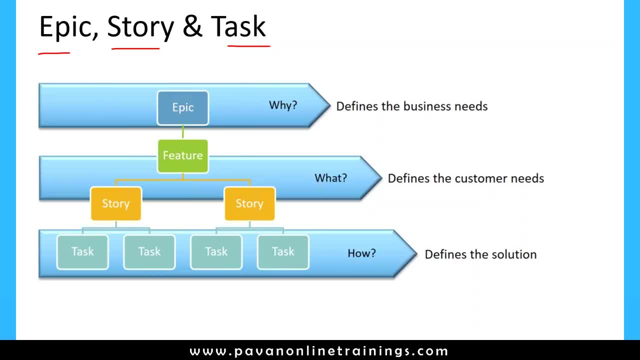 Okay, So everything will happen very faster. So if you create for everything, if I created some document, it takes a lot of time right. So the document 90%. the document will be avoided in agile process. So here we don't have any FRS document. 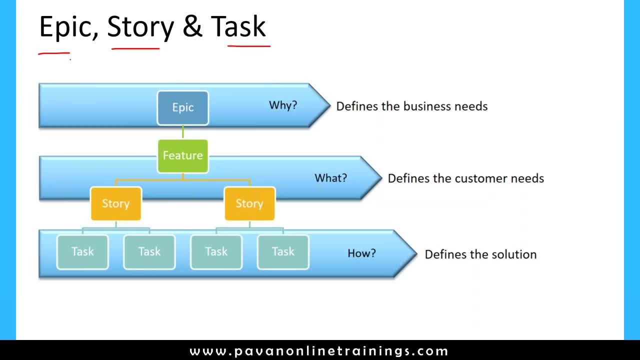 to understand the requirements. So instead of FRS document we have epics and stories. So what is epic and what is story? So epic is a larger requirement. So basically it is designed by by means, define the business needs. Let's say there is a customer. 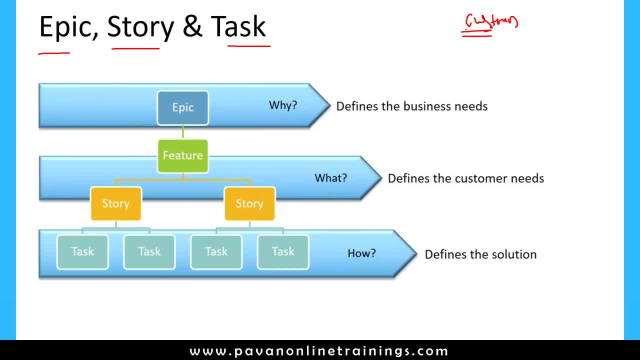 So he will create epics. So what is their business requirement? And they will create, set a number of epics And based on this epics, epic is nothing but a larger requirement, very high level and very larger requirement. And based on this epic, 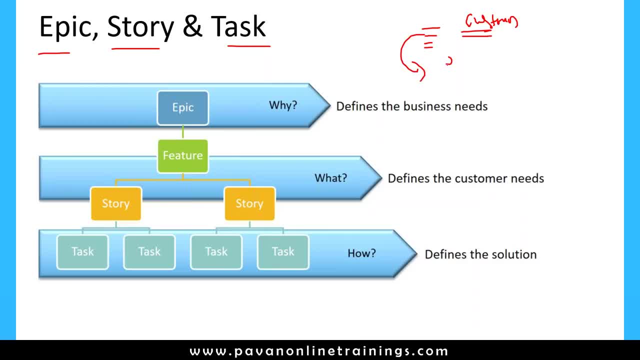 we have to derive these epics into smaller pieces. They're called as a features, again divided into number of story. So story is a nothing but a smaller requirement. Story is nothing but a smaller requirement And epic is nothing but a bigger requirement. 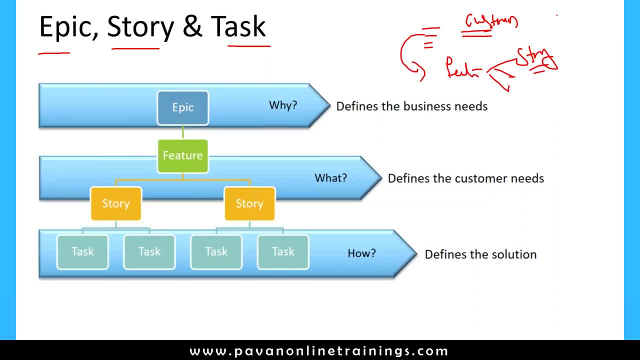 a larger requirement, okay. So, for example, let's say, one epic is there. So let's say, as a suppose, as a user: okay, I want to use online banking application. So, as a user, I want to use online banking application. 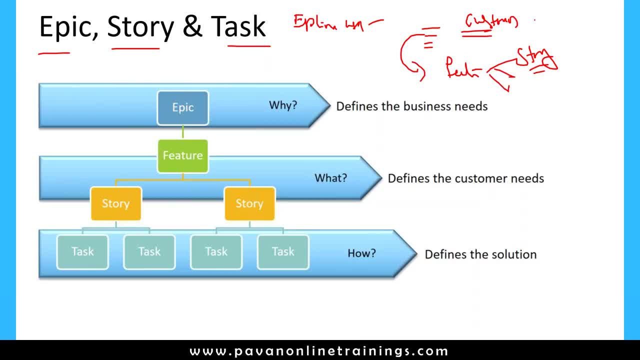 So that is an epic. There's a very bigger requirement, right So, as a user, if user want to use online banking application. so there are so many functionalities and scenarios to be there Again inside that particular epic if I divide it into multiple pieces. 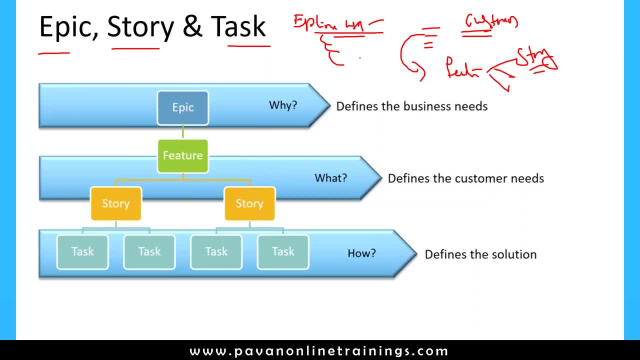 as a user, I need to log into the application as a user, I need to verify my balance. as a user, I want I can send a transfer, I can transfer money. So these are all activities we can do. So all these things are comes under the stories. 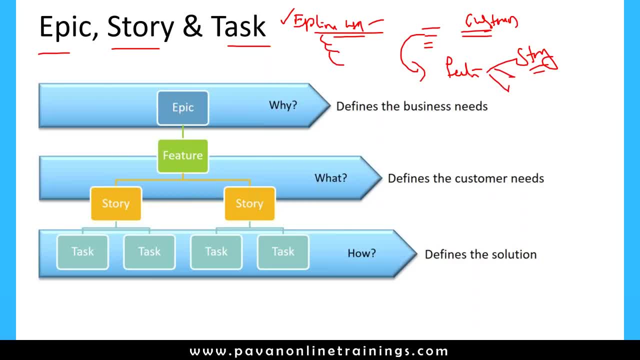 So epic is a larger requirement, whereas story is a smaller requirement. And if I divide epic into multiple pieces, that's okay. And if I divide epic into multiple pieces, that will become a story. So that means define a customer needs. Actually, the story is talking about detailed requirement. 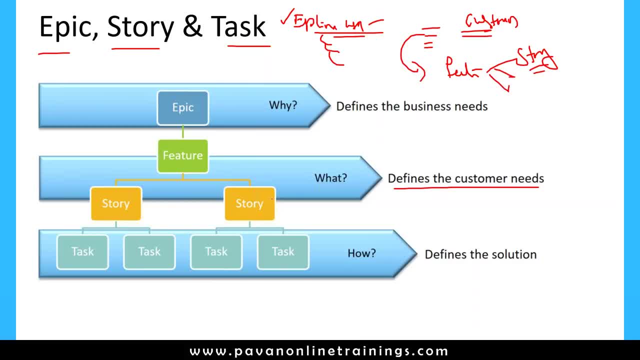 So by understanding this story, by reading this story, we can understand the functionality of the application. Okay, so in agile process we don't have any requirement kind of stuff. We have only epics, as well as stories, features and stories. 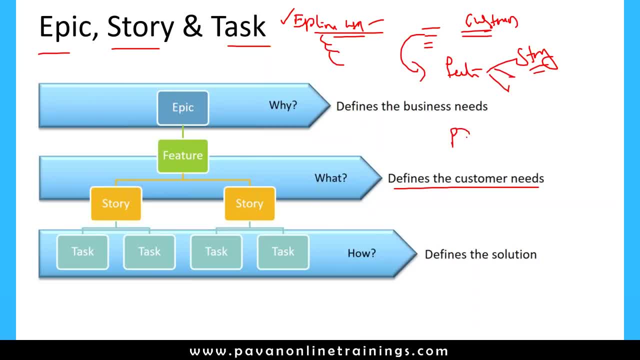 And who will derive this? These are all derived from product owner, So there are some different designations we have in agile process We are calling as a product owner, scrum master, agile team stakeholders. There are a new terminology is coming to the picture here. 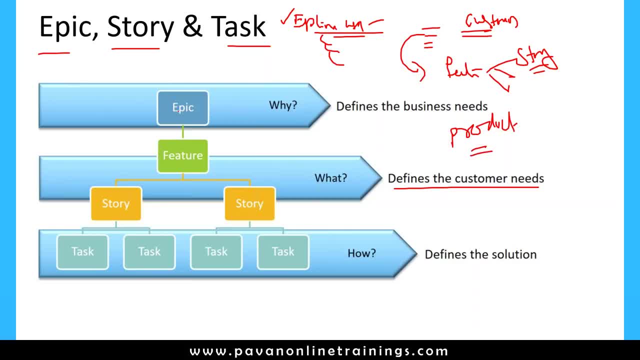 Okay, now here, who is responsible for getting these epics, stories and all means? product owner is a responsible guy, Who is responsible for get this stories and create these stories based upon the features which are provided by the customer. Okay, so this product owner is a main person. 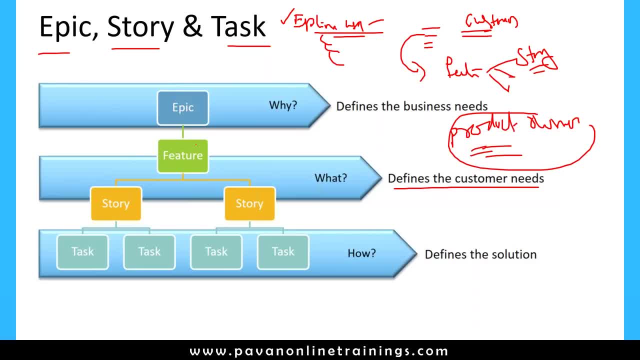 Who is always in charge of getting these stories? We are calling them as a product owner, Agile team, stakeholders with the customer. so he has to get all these features as well as stories from the customer and he will prepare these stories, will get the feature from the 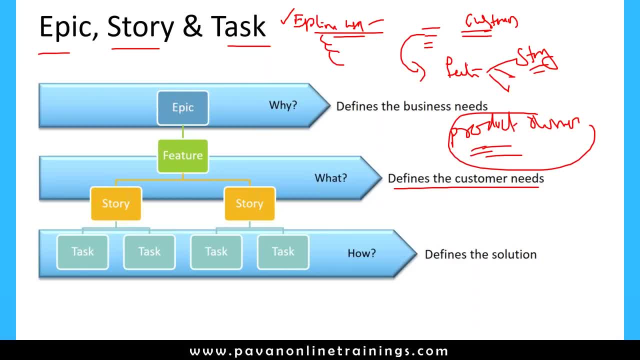 customer and then he will prepare a stories for all the features and all the epics. he will create all the stories. okay, and these are the input for us. so if you want to understand the functionality, we need to understand the story, we need to go through all the stories. the story is a, a smaller, 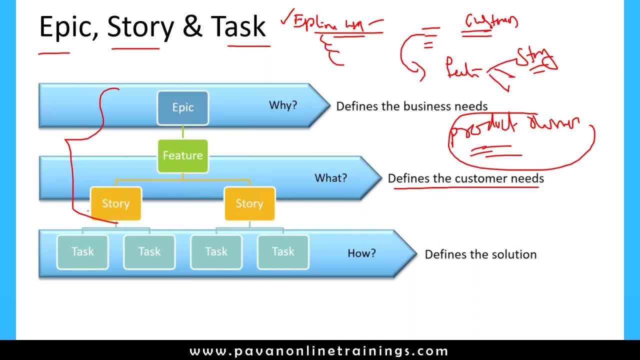 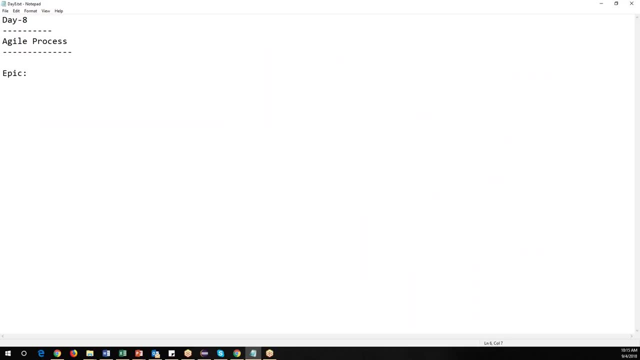 requirement in a gel process. now for that particular story, we have to create number of tasks. so, for example, let us say an example. so for example, here I'll just create one epic. let's say I have an epic like this. so what is an epic is a. 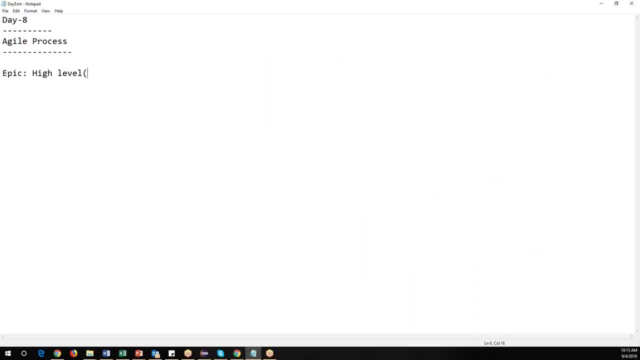 pic is nothing but a high level requirement. high level or is a huge requirement? okay, so example: so as a user, I need to use online banking application, so this is an epic is a bigger requirement. so, as a user, if you want to online banking application, I can do a lot of things on this, but this 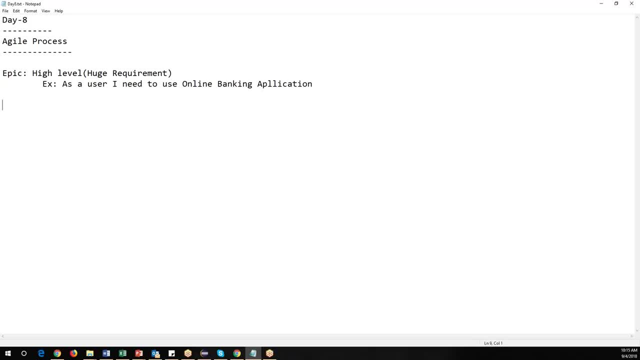 is very high level requirement. this is called epic. now let's say story now. so story means it's smaller kind of requirement. let us say, as a user, this is a story. as a user, I can login into online banking application. so this is a one story application. so this is a one story application. so this is a one story. 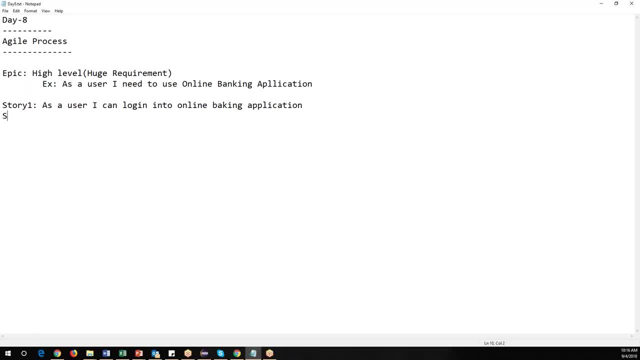 we have to. and let's say, you can safe, you can get multiple stories like and story two. so as a user, as a customer, I can verify or I can check. I can check my balance on my balance in my account. so this is another story. so, like this, we 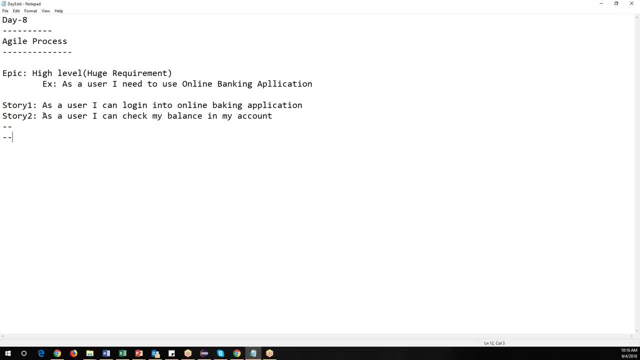 can create any number of stories for this epic. now, every story contains but specific number of tasks. So let us say, take this particular story, So this story for this particular story, tester will work on it and developer is also will work on it, parallelly. 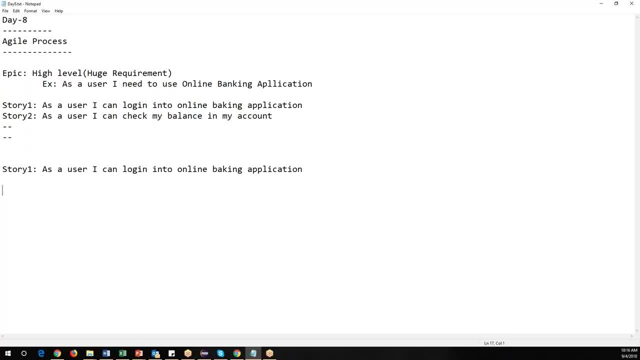 So what developer will do here, this particular story? what are the developer tasks they has to perform? So developer has to perform certain things on this particular story. So what they will do is they will understand this story or they will review this story first. review the story and they will estimate this: how much time this story will take for development. 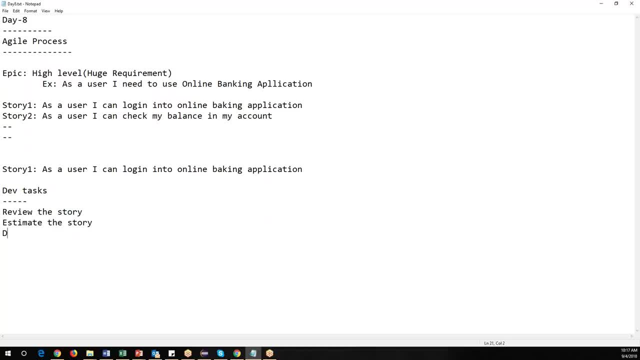 So they will estimate the story and they will design the story and they will develop or they will code it right, They will code it and they will perform unit testing and integration testing. So these are all comes under the development task for this particular story and similarly, parallelly, QA also will do their own task for this story. So, for example, what 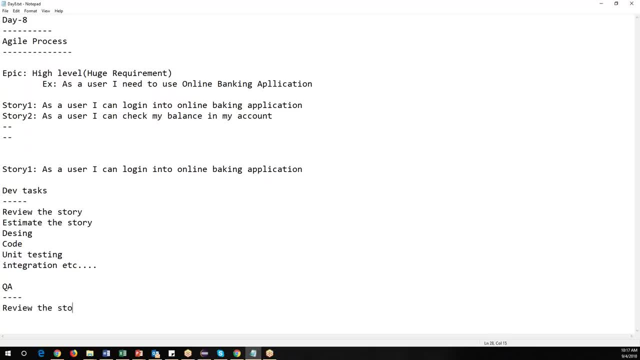 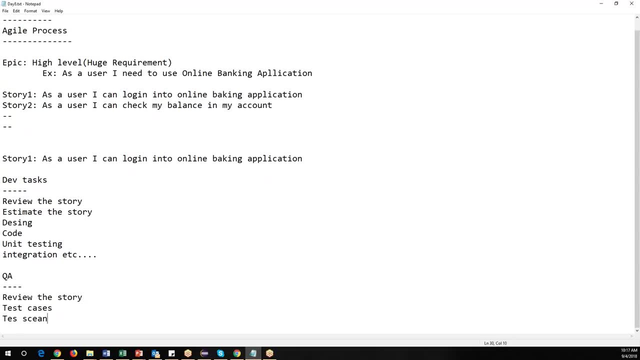 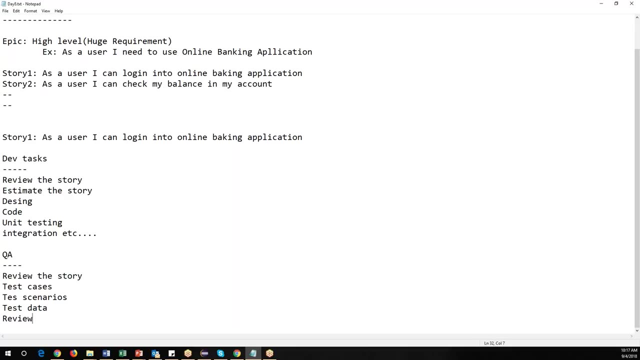 the QA task. The QA should also review the story- What is the story? and he has to prepare the test cases and test scenarios for that particular story, right, and he has to prepare the test data for that particular story and he has to review those test cases with the team. and 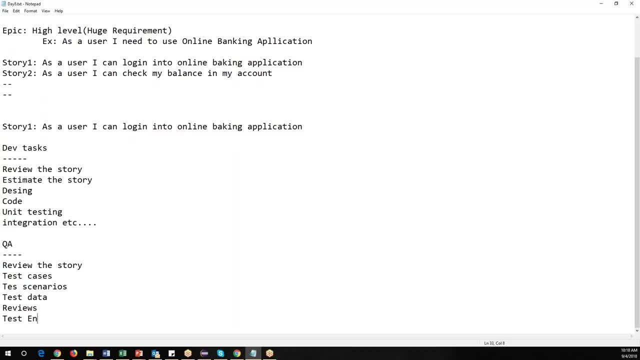 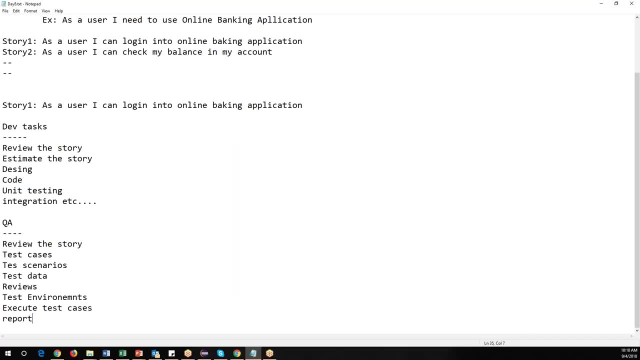 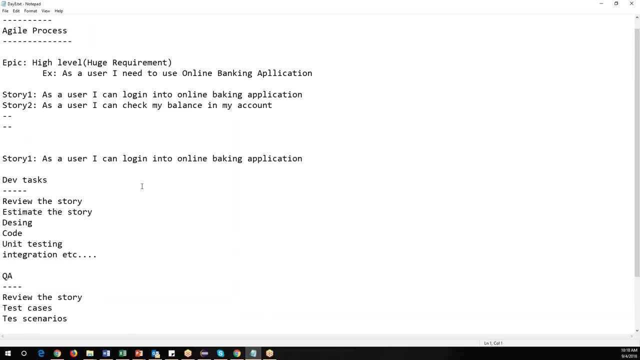 he has to prepare the test environment and has to execute your test cases and he has to report the bugs. So these are all comes under the testing activity, These are all comes under the testing. So what we understood we so far is in agile process will start with the epic. 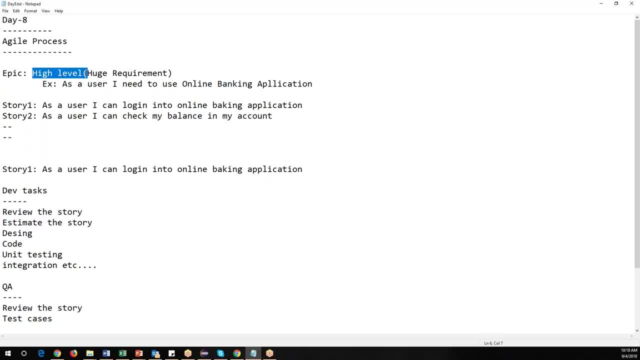 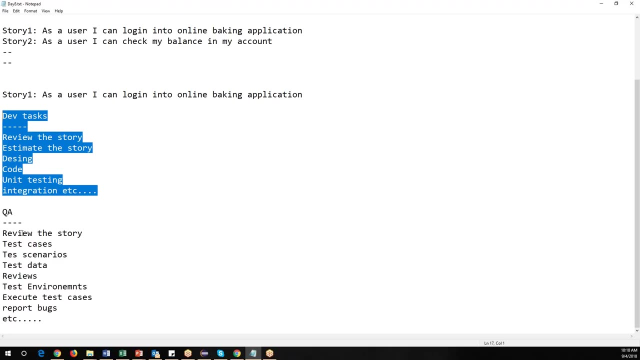 So epic is nothing but very high-level requirement from the customer. So the product owner will divide these epics into multiple stories- a smaller piece of requirement- and for every story the developer will perform certain tasks, and for every story, QA also will perform the their own task. 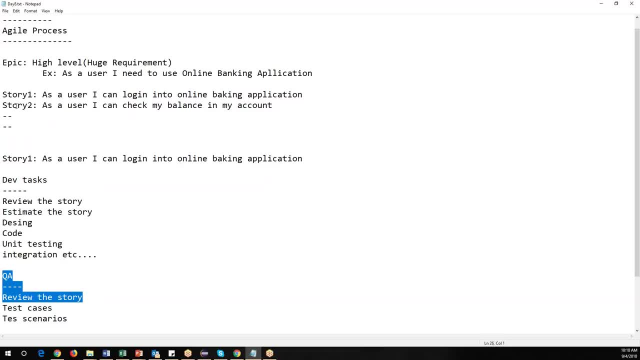 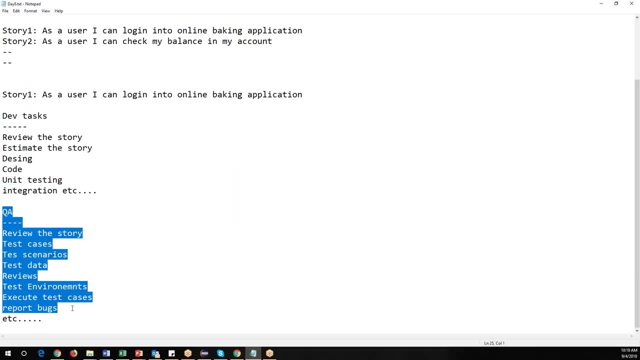 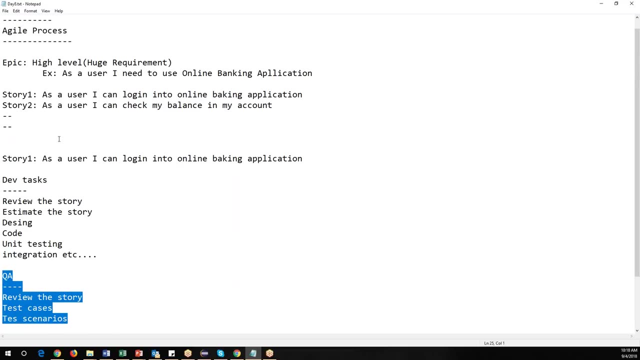 So collaboratively, the dev as well as QA will work regarding this particular story. So once the story is completed is nothing but the development activities and also QA activities will be completed, and then only we can say the story is completed. So once the story is completed, we will demo it to the customer again. 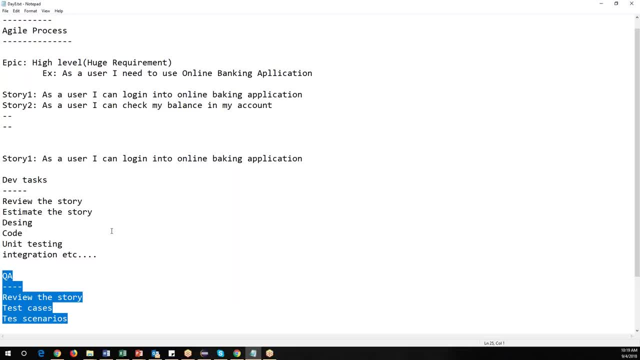 So first we need to demo it to the team QA, dev as well as product owner, and then we will demo that particular story to the customer. Okay, if the customer satisfied is fine. Or if he see, if you suppose, if the customer say some more changes, we can just accommodating. 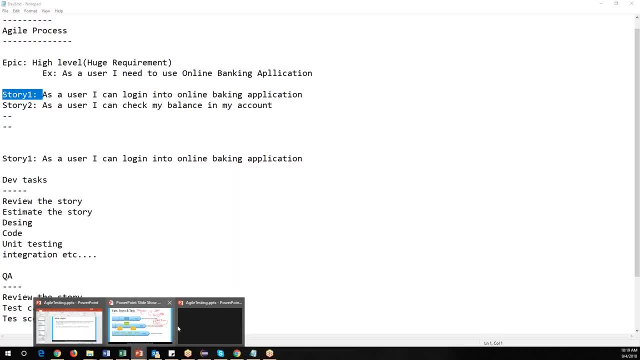 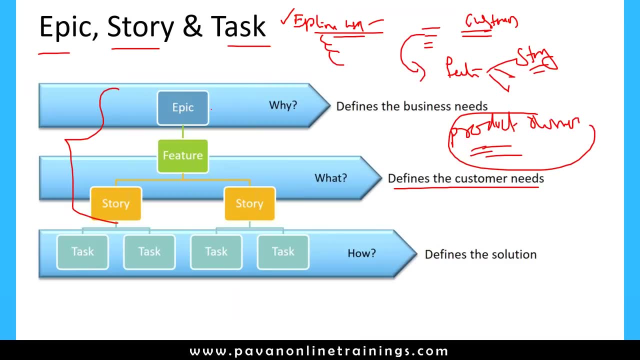 it Okay. So this is how we need to process. So first thing, in agile process, we need to understand what is a big, what is story and what is the task. So epic is a larger requirement and stories of the smaller requirement, and the task is. 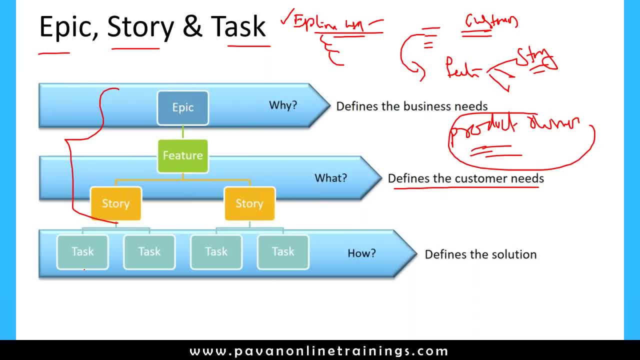 an action which we need to perform on that particular story. Okay, and what is the difference between product owner and business analyst? So business analyst basically comes in the previous For model and other models we call as a business analyst, So he will analyze the business, basically. 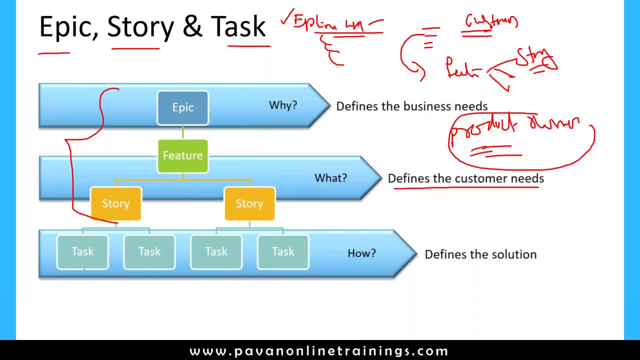 Okay, Yes, in the agile process We don't have any business analyst and also we have only product owner. Okay, product owner is a responsible for getting the requirement from the customer and here we don't have any kind of business analyst guide. So business analyst is a role or designation which will comes under the waterfall or other. 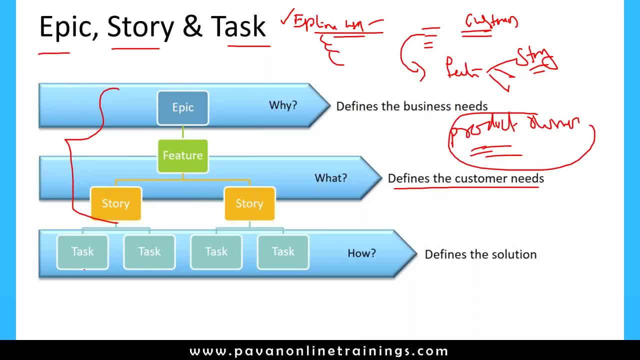 other models, like we model and other models, but here we don't have specific designation. Product owner is a responsible guy, So we is interacting with the customer always okay. So product owner is also a guy, So he's a person, he's a responsible for getting the requirement from the customer. 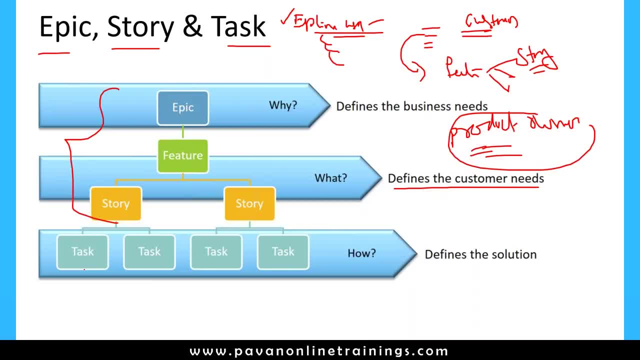 So I'll talk about those responsibilities. Okay, just wait for a moment. fine, So here we are. meet. we have to understand first what is a big and story and tasks. So we have understood what is a big. it is a larger requirement and story is nothing but. 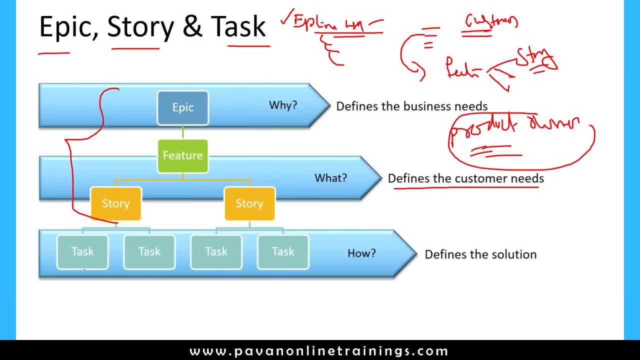 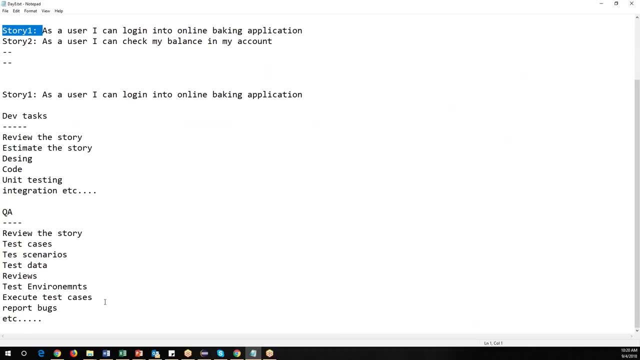 a task. Okay, It is nothing but a smaller requirement, and task is an action which we need to complete for that particular story. Okay, Now let us move on to the process. So here I have listed out the rules. So, especially in agile, there are three different roles. 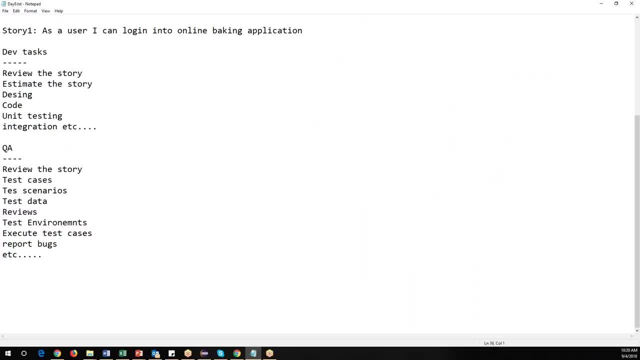 I'm not talking about classical models, Okay here, just remember, these are the rules we have in agile roles. So the first person in the agile process is a product owner, So he is the person responsible for getting the requirements. getting the requirements, So he is the guy he's always interacting with the customer. okay, 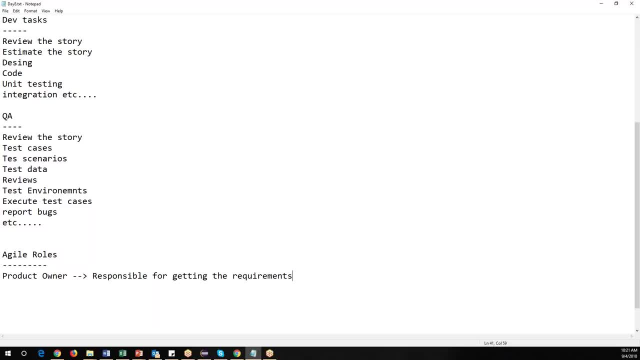 So product owner is a responsible for getting the requirements. the product owner means he is not a customer. Okay, He is not a customer, So he will get the requirement from the customer, requirement from the customer, and also call, as a stakeholder, Stakeholders. 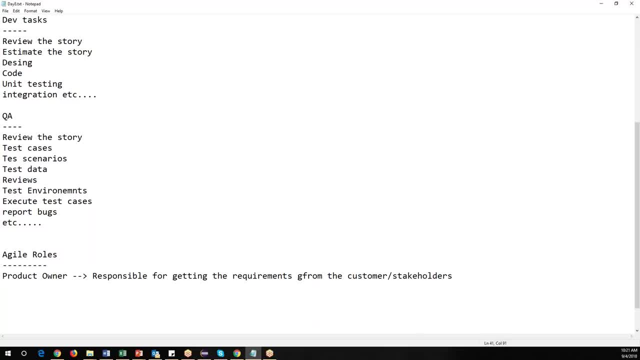 Stakeholders are nothing, but they are the people will use the software later. So product owner owner is the first person, is a mediator between the company as well as a customer. So he is a responsible for some, will get there all the requirements and also he will do a. 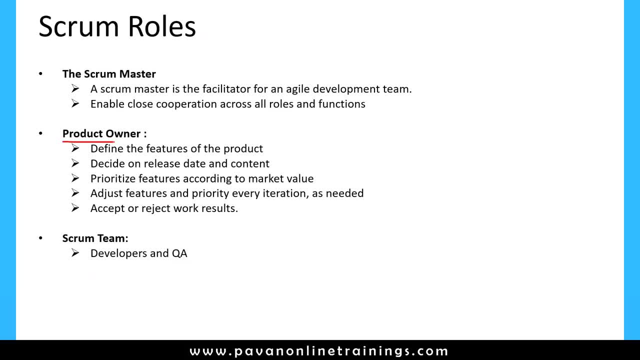 lot of activities. So what is the responsibilities of product owner is he will define the features of the product. So, based upon the customer requirements, he will define the features- features on the sense- again, epics and stories- and he will also decide on release date. 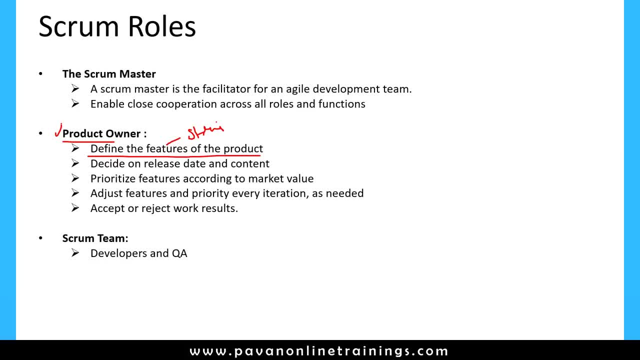 Okay, So he will. he's the person who will decide the release date and everything, and he means the person will prioritize the features according to the market value. So suppose the customer given a, let's say, 10 requirements and the product owner will decide which one is a priority one and those features will deliver first to the customer. 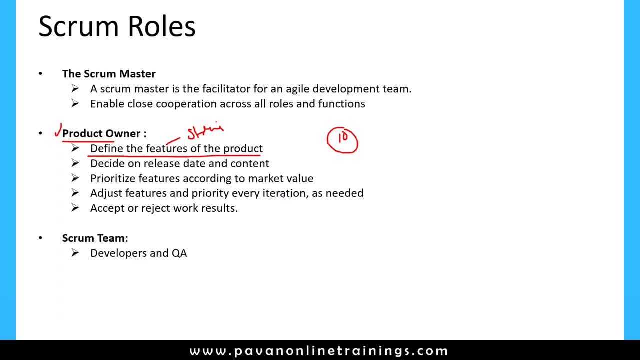 and he will also responsible for adjust features and priority every iteration as needed. So sometimes initially we got 10 requirement from the customer and product owner is responsible For what are the first features we need to deliver, because we don't deliver all the features at the same time to the customer. 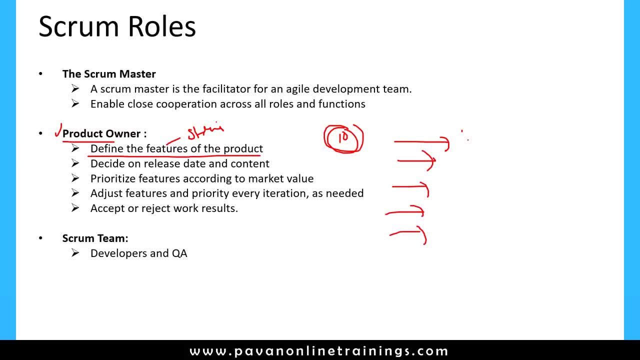 So we will deliver them in version by version. in the first version will deliver few features. in the second version will deliver few more features like this. So what are the features? we need to go first. So that is again depends on this, decided by the product owner. 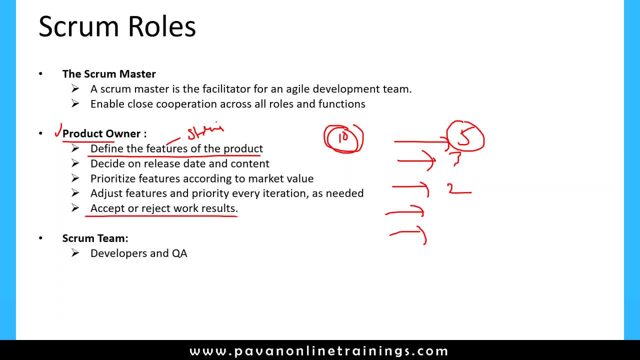 Okay and accept or reject the work. result: Suppose a developer as well as testers work together and then completed their development and testing. Finally, they have demoed the product to the owner. product owner and product owner should decide whether the okay- the product is working according to customer requirement or do we? 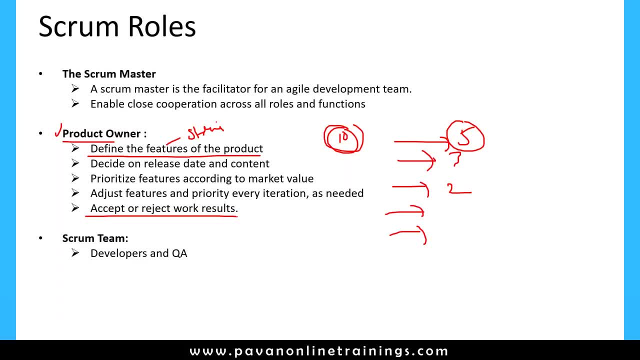 need to do certain changes. So if he is not satisfied, you can just reject it, and if he is satisfied and then we can deliver to the customer. So these are the different roles the product owner will perform. Okay, So he's main role is getting the requirements from the customer, creating the epics and stories. 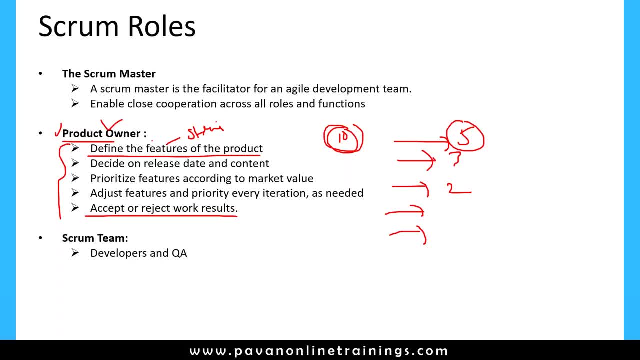 and prioritizing those stories And deciding the release dates and all. and then he is also a have right to accept or reject our work results. So these are the main tasks the product owner will do. Okay, these are one guy in the agile process and along with this product owner, 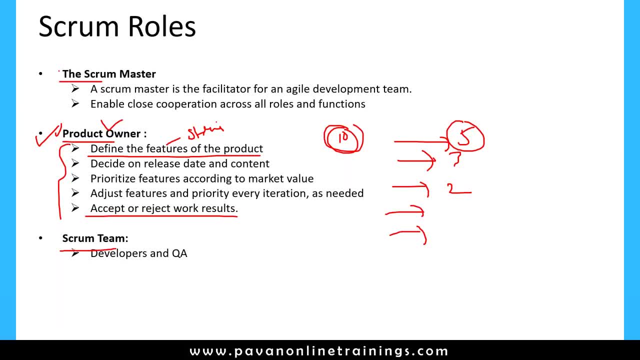 We have also scrum master and scrum team, So scrum master is a different role actually. So scrum master is a, not a manager, is a not a developer, is not a tester. Okay, he's not belong to any specific team. 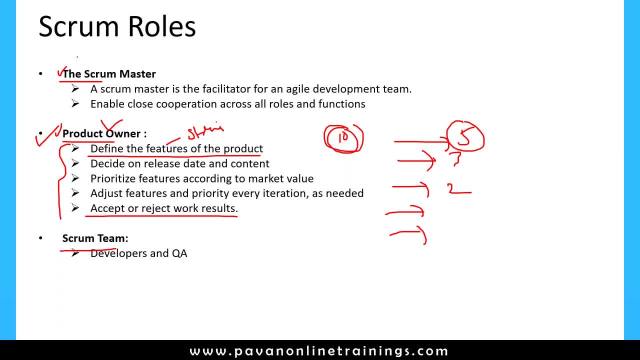 So scrum master- He's a specific role- who is facilitating the complete agile process, all who is driven the complete agile process and also scrum master is not owner of the product. You don't care about the product, you will care about the process. 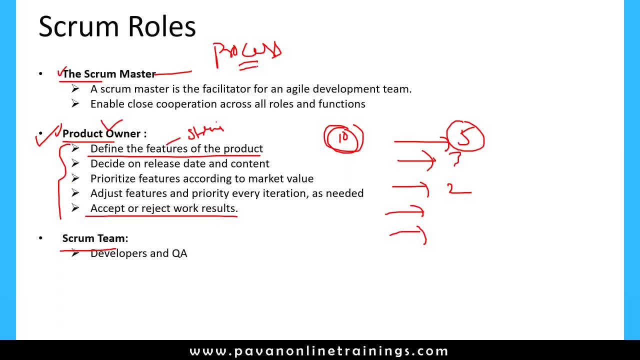 Okay, It's a scrum master is always talk about the process, how work is is going on. Okay, Is there any blockers? how we can proceed, What are the challenges we face and how we can overcome these challenges. So all these things are taken care by the scrum master. 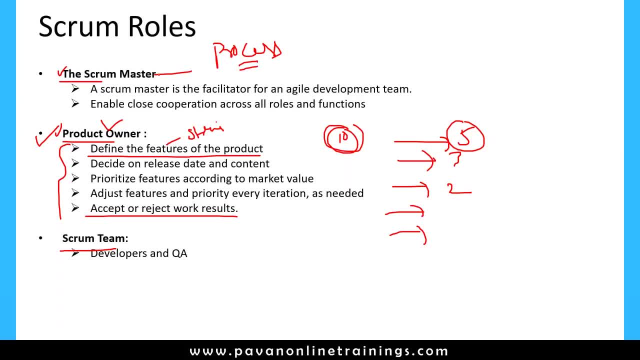 And remember this: scrum master is not a developer. scrum master is a, not a QA or tester. scrum master is a, not a manager. Okay, scrum master is a different role. So normally in the company's over is having, or who is done the scrum master certification. 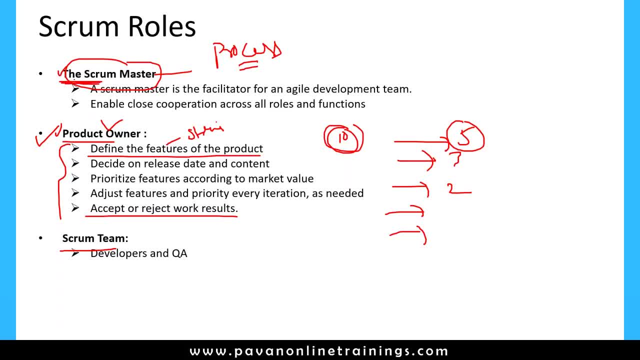 So they will recruit those persons in the scrum master role So they will drive the complete agile process. Okay, and he's a mediator person between all the team: product owners, developers and QA everybody. So scrum master is always a developer, Okay. 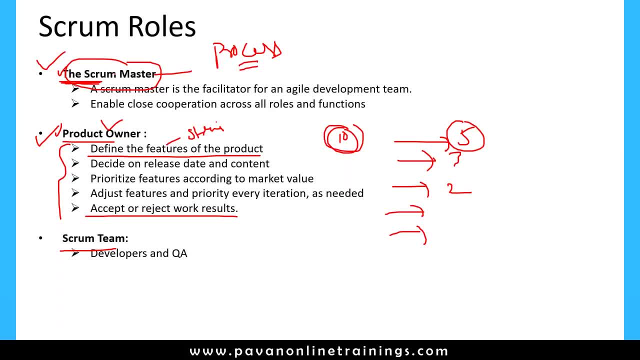 He is also very important person in the agile process. He can drive the agile process, and the other one is a scrum team. scrum team is nothing but developers plus QA, So all comes under the one team because they together will work for one goal. 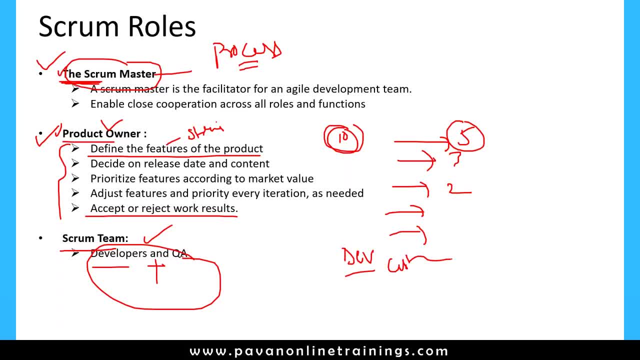 So what is the goal here? We need to deliver the product to the customer. There's a only one goal, So to deliver this particular product on time. developer, as well as testers, should work. So these are the. these people are Actual executors, actual workers, but product owner is responsible for giving us the inputs. 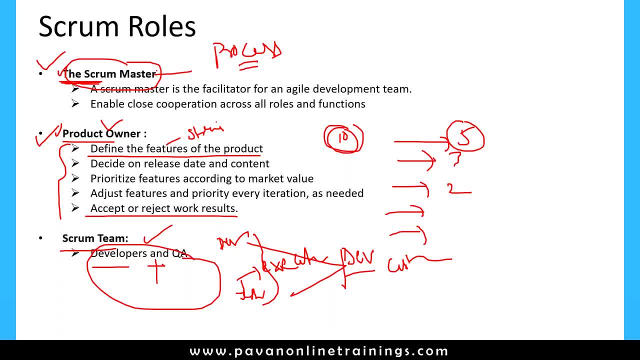 from the customer and scrum master will drive the process, complete agile process. He will drive it. Okay, That is the role of scrum master. So scrum master, product owners come team. So other than this role, there is no other role present in the agile process. 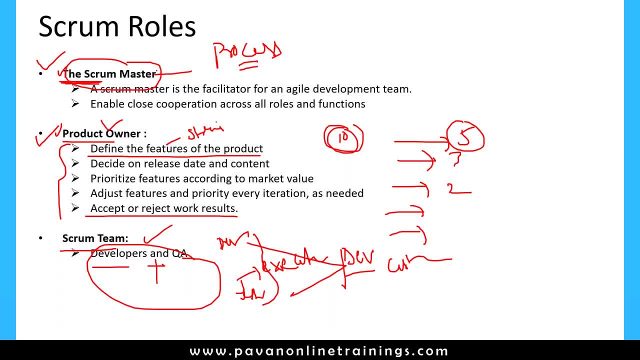 So business analyst or technical and other people are managers. do manager QA manage the resolve Like people management okay, not for the product, okay. So especially for agile process, we have only three roles. One is scrum master, product owner and agile team. 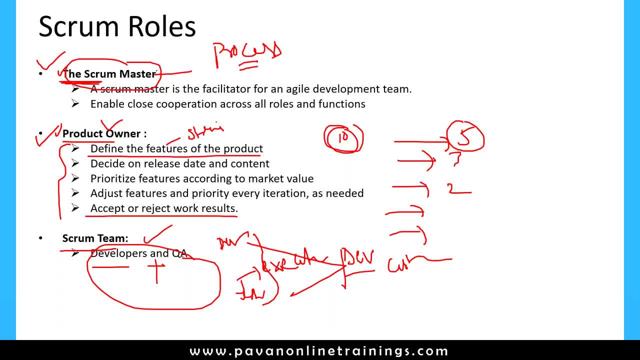 So agile team in the sense, and developers as well as QA, okay. So this is the first and very important thing we need to understand now. So, before going to process of agile, we need to understand two things Here we are talking about. 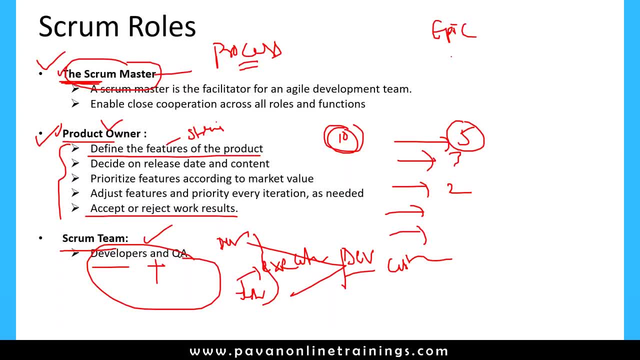 Epic, right, Okay, And there we talk about the what is story and we talk about what is task. So epics are divided into multiple stories and every every story, the developer is having his own task and the QA is also having their own task. 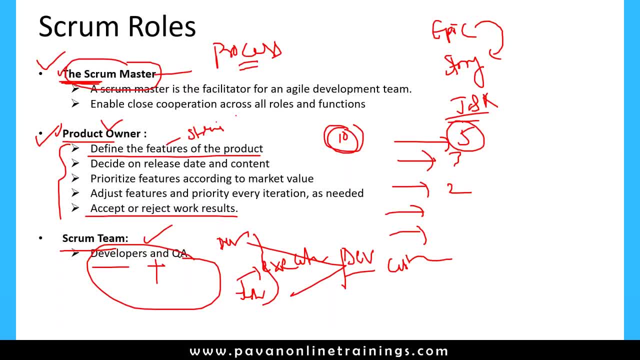 And here there are two things we need to understand. that is uh D O R, okay, And there is other one: definition of done. So D O R is nothing but definition of ready And uh D O D must a definition of done. 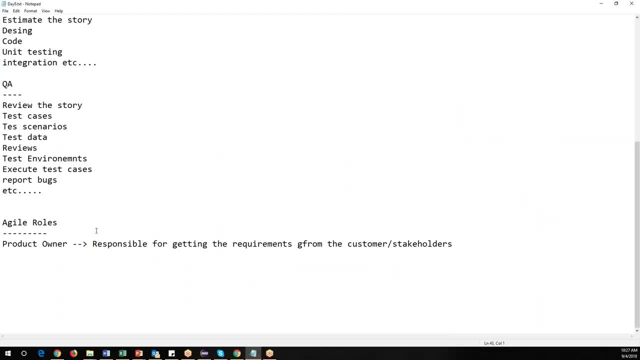 So these are the two things we need to understand. Let me just write it out: D O R means definition of ready and D O D means definition of uh, definition of done. So these are the two terms we need to understand here. 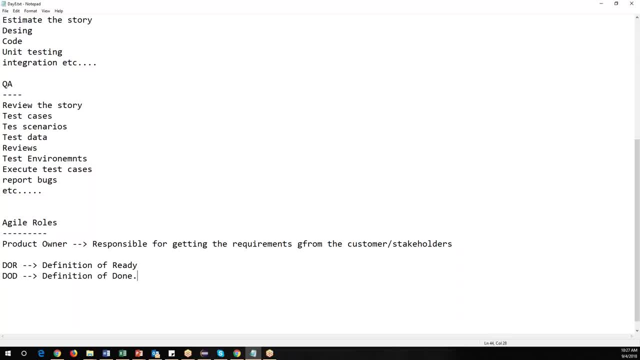 Especially in agile process. D? O R means definition of ready and definition of done. So if any activity, if I do something, suppose if there is a story, let us say, one story is there. So when we need to say whether the story is ready to pick up for coding and testing and 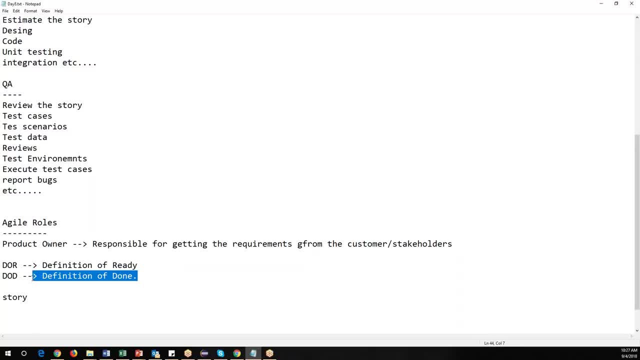 when we need to say whether the story is completed or definition of done. So we need to follow certain rules here. So any task, it can be story, or it can be epic, or it can be document, or it can anything. If I say something, you will tell in the status report you will say: okay, I have done something. 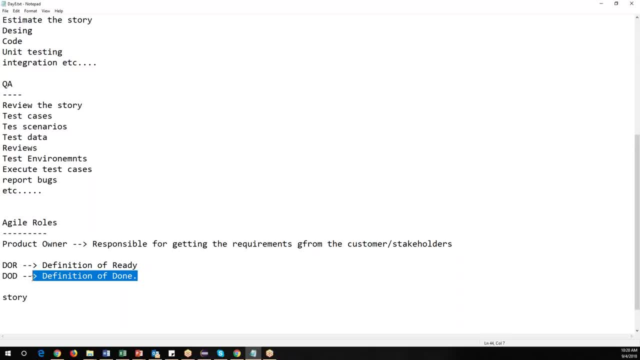 So what is the meaning of done? So, when we need to say what is done? and, similarly, what is the definition of ready? Suppose, uh, they say like story developer says like okay, story is ready for testing. So what is that ready? 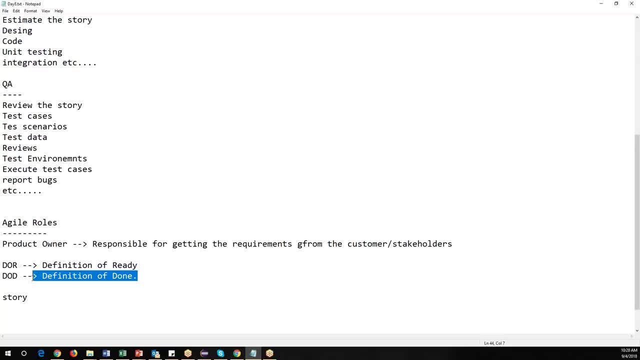 So what is the criteria we need to have to make that particular stories ready? And similarly, if I say story testing is done, so what is the done means when we need to say the story is done, So for that we need to have certain rules here. 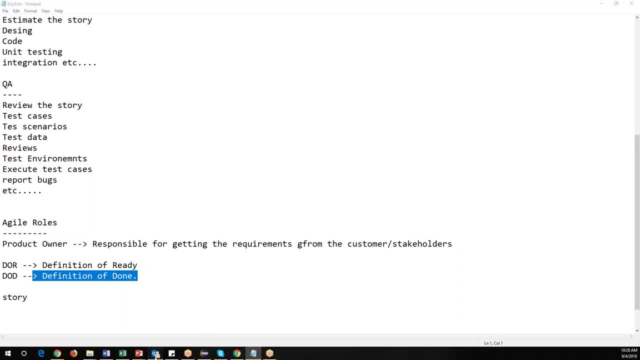 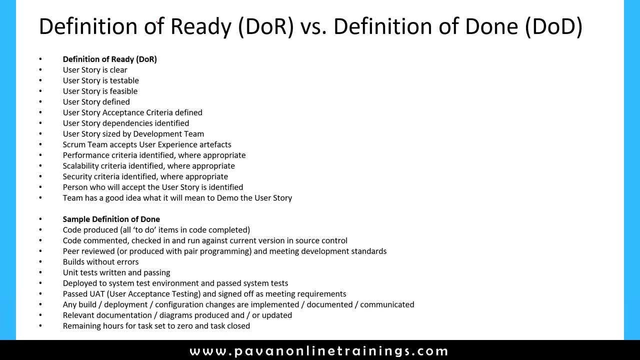 Okay, We need to define certain rules in the agile process. Now let us discuss those rules here. So definition of ready and definition of done. So when I say definition of ready, we need to have certain rules like: user story is clear and user stories testable user stories, feasible user stories, defined user story acceptance. 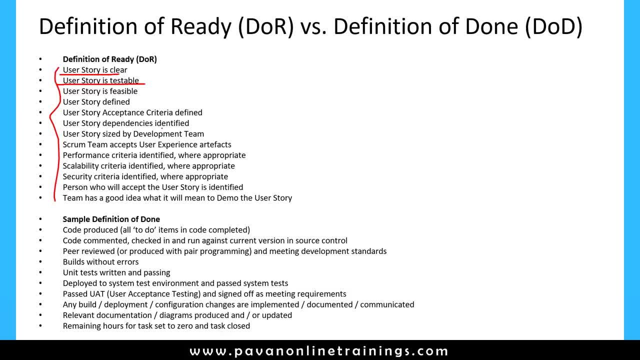 criteria defined, user story dependencies identified and a user story dependencies are identified, No User story size by development team. So once we reach all these things, once we are done all these things, then we can say: particular user story is ready for uh testing. 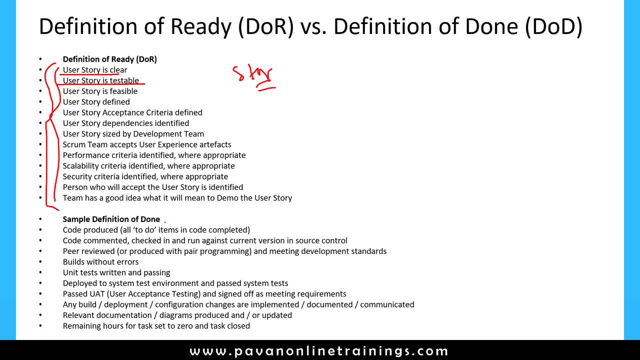 Okay. And similarly, if I say definition of done means when we have to say a story is completed, means what should be produced for is commented, checked in and against current version in the source control: peer review: bills without errors, unit test, return and passing deployed. 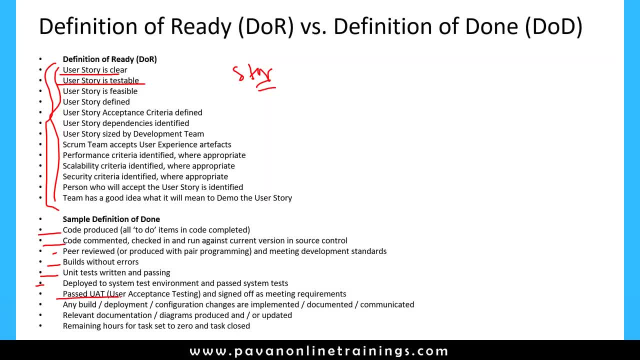 uh, to system testing. I'm going to pass a system test and pass you 80 test, Okay, So all these things should satisfy, and then only we can say definition of done So when a task or a story, if I say it is ready for testing, or if it is ready, then 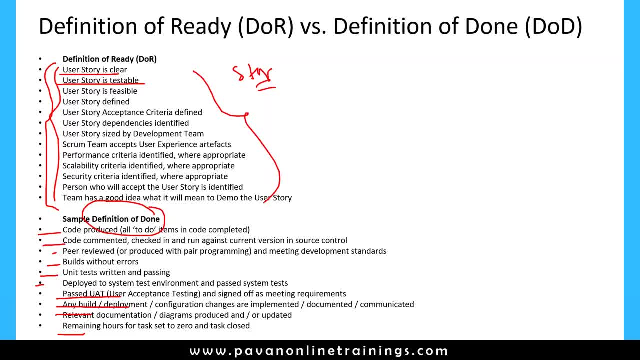 it should satisfy all these points. And if a something or, or it is a task or story, if it is done means it should satisfy all these rules, but all the rules not applicable for all the times, but at least we need to follow these particular rules. 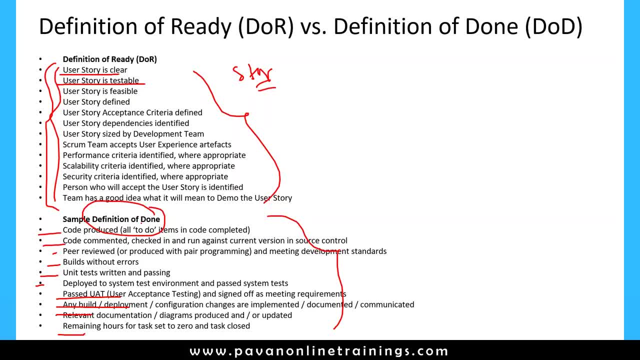 When I say done, Okay. So before jumping into the agile process, we need to understand these terms. What is D O R? What is D O D So? D O D D O R means definition of ready means. it is a number of rules which we have designed. 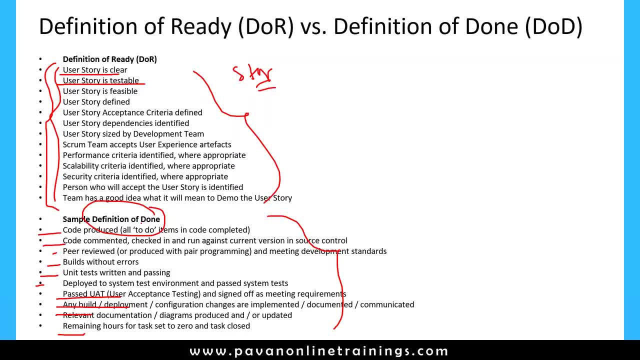 Uh, when we say a story or task or APK is ready, And similarly definition of done means it is- contains a set of rules which says about when we need to say done Okay, Before when I say something is done, We need to cross verify whether all activities have been completed or not. 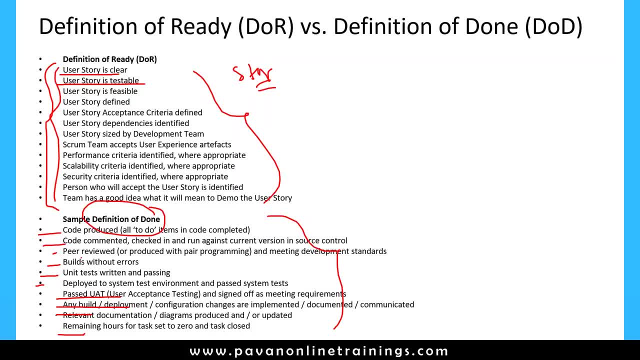 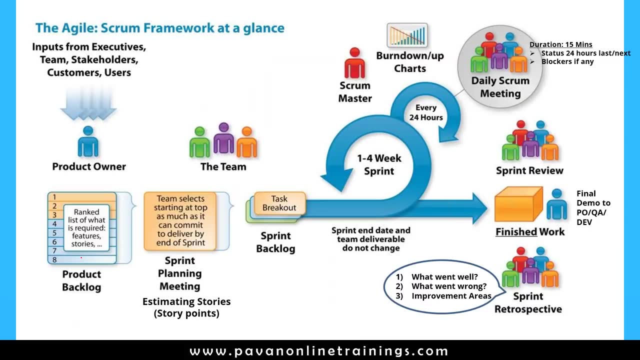 And then only we say, okay, we have done. Okay, So this is all about definition of ready, definition of done. So this is just theoretical understanding you need to have beginning of before jumping into the agile process. Okay, Now let us discuss about the complete process, end to end process of agile. now 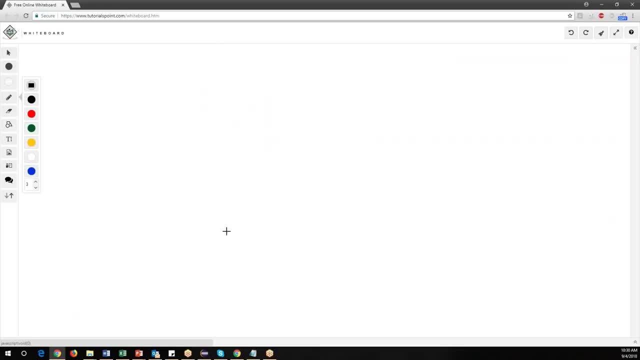 So let me just tell you a very high level first, and then we'll go to the picture. So suppose the customer- Okay, So the customer we have, let's say a customer- Okay, So here we have a product owner- is a product owner. 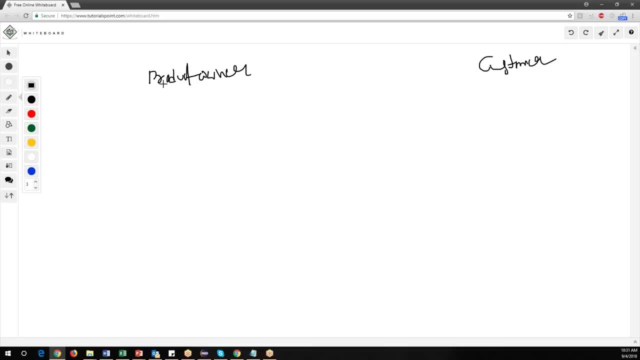 Okay And uh, we have some master as well as a jail team. So first, how the planning will happen is, initially, the customer is having some APKs and the product owner will get all the information from the customer. and a product owner will have uh, 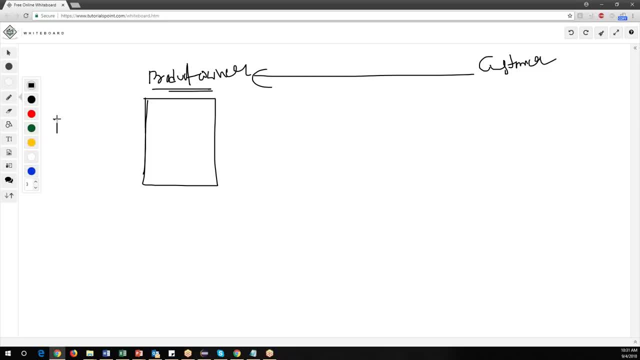 we'll prepare some uh document here, So this is called as a product Backlog. Remember this. Okay, This is called as a product Backlog. These are the new terms which we need to understand. So what is the product backlog? 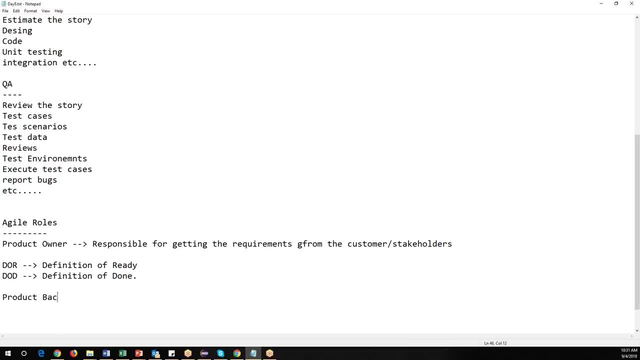 I'll write it here: Product backlog. So what is the product backlog? product backlog, in the sense, this is a uh prepared by, prepared by product owner, and what it contains, which contains requirements, which contains requirements. So product backlog is prepared by the product owner at the beginning level and uh which? 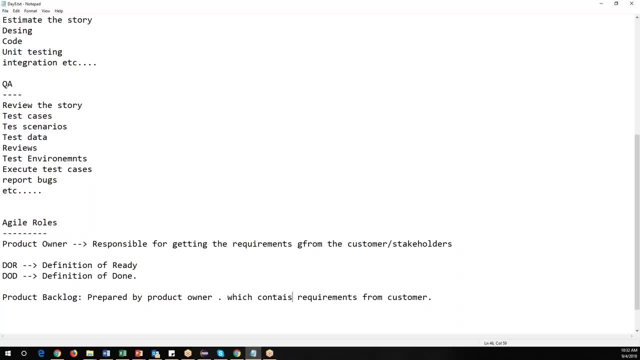 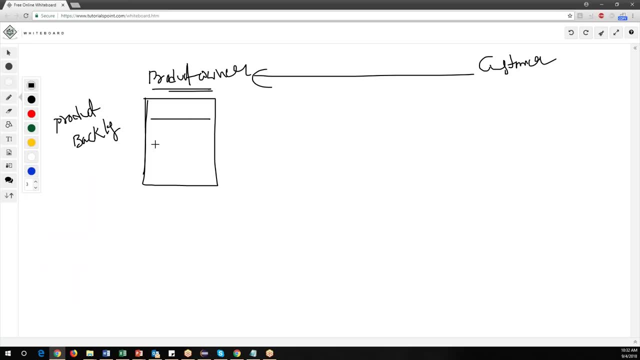 contains the which contains the requirement, contains the requirements which are given from the customer. So this is called about product backlog. So product owner will create the product backlog, So which contains the all the requirement. normally it is an Excel sheet, Okay. 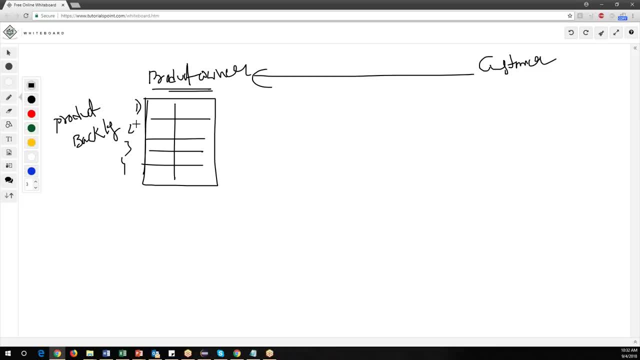 So you will note it down: one, two, three, four and everything. So this contains the requirements in the sense stories- Again, a big sense stories we have in this document now based on this. So the complete team, like product owners, scrum master, agile team, will have a meeting. 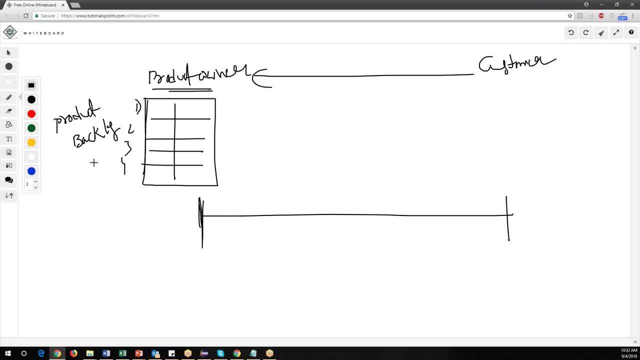 release planning meeting. So this is complete release process. Okay, So let us say he has a 10 epics or 10 stories have to implement, So they don't provide all 10 stories at the same time to the customer. So let us say customer wanted all the stuff. let us say within three months, this is the 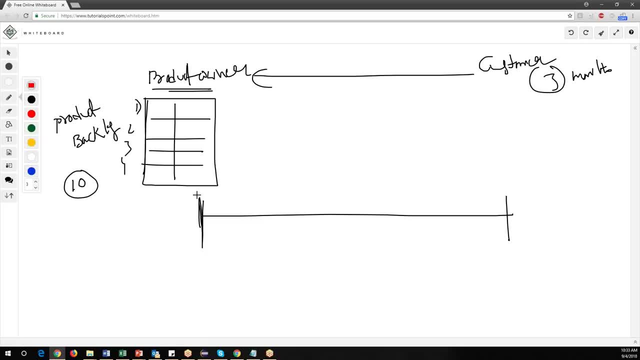 time Now within the company. So in the release planning stage, what we do is the complete. we have a three months of time. So three months of time completely divided into multiple parts. Let's say I have 10 features or 10 stories. 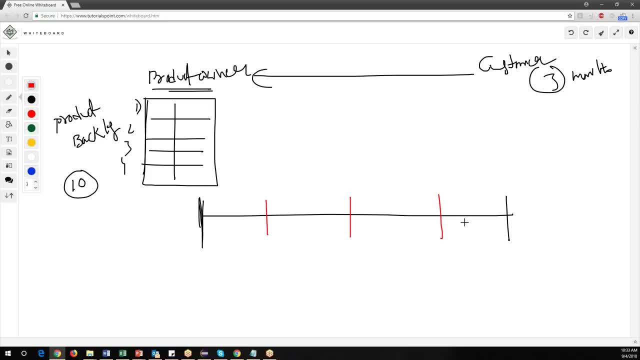 So we will divide entire cycle, or three months, into multiple parts, and each and every part is called as a sprint. This is called as a sprint, or we also call it as a iteration sprint or iteration. So it will be normally two to three weeks, not more than that. 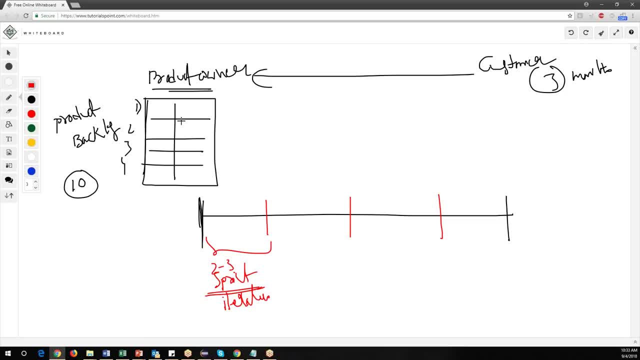 Okay, It will be two to three weeks of time Now in the product backlog, whatever stories we have, so product owner will prioritize them. Okay, They will prioritize them. Which are: what are the stories we need to implement and test in the sprint one and what? 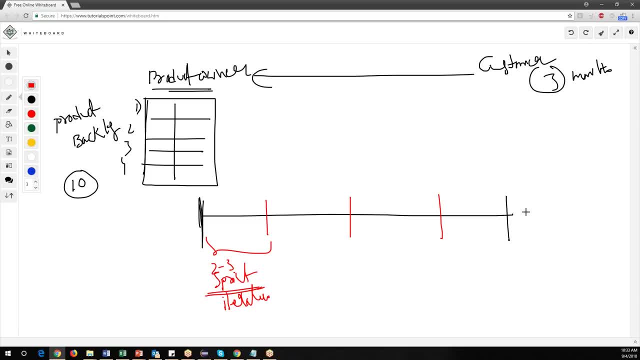 are the stories we need to implement and test in the sprint two and sprint three and so on. So in the first sprint, let us say: three requirements have implemented and test implemented. test means we have to complete that, Okay. So once we completed the first sprint, one version of the software released to the customer. 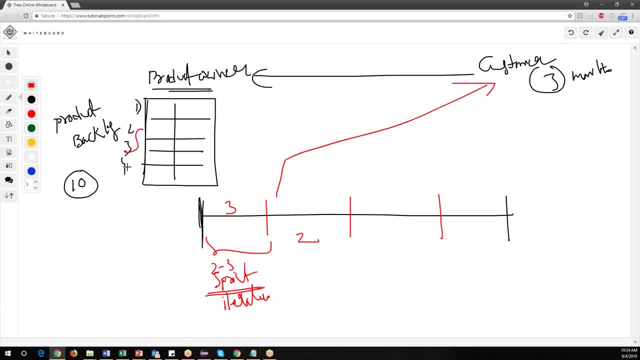 and on top of it again we'll start the second print and again we'll take few more requirements on few more stories and development and Q activities will going on And once the second print is completed, another version of software released to the customer. 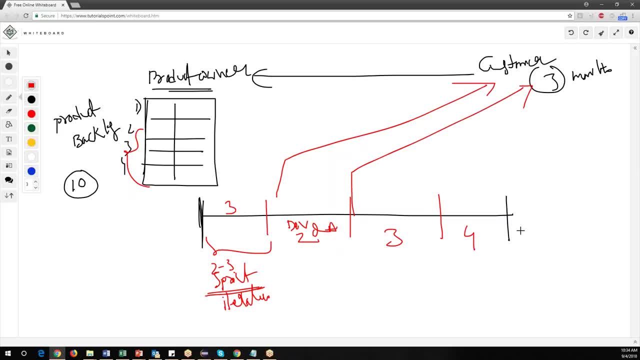 and similarly sprint three, sprint four. At the end of the last sprint, the complete software will go to the customer, because by that time, all the stories have been developed as well as tested. Okay, So this is how the agile process will happen. 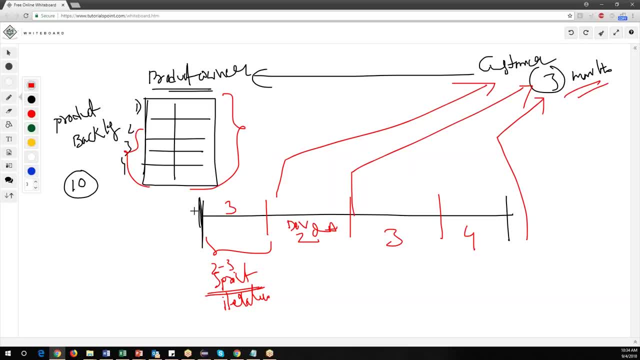 So it very highly well, the release time will be divided into multiple sprint and every sprint we need to plan again. So this is the main activities we do during sprint. Okay, So every sprint, developers will do certain activities and testers will do certain activities. 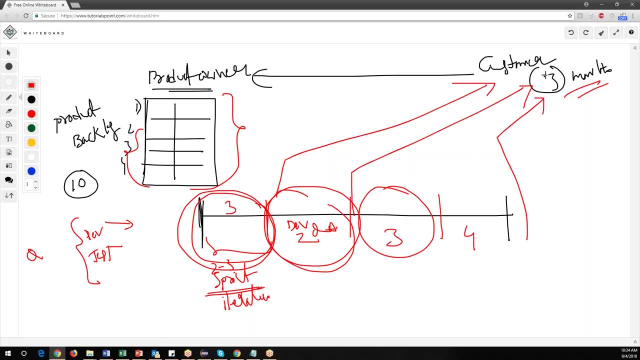 and before that we need to also do the sprint planning. So release planning is different And sprint planning is different. In the release planning, all the team will decide how many sprints are required and each sprint how many stories we have to develop and test. 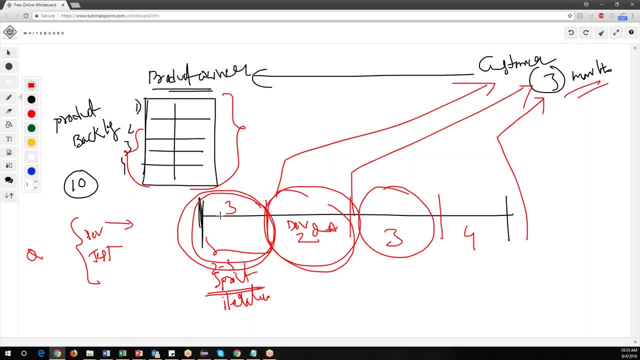 But in the sprint planning we have to decide what are the stories we have to develop and test and what is the duration of the print and what are the different tasks the developer will do. What are the different tasks tester will do? What is the estimation? 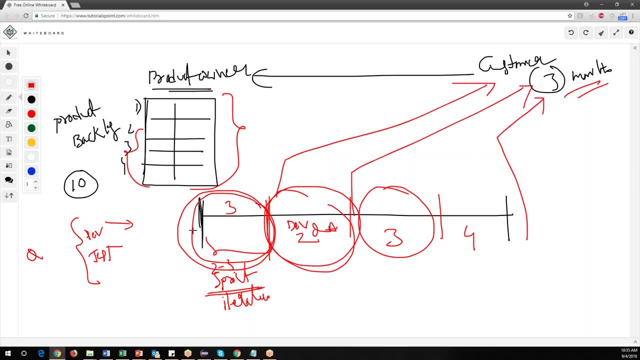 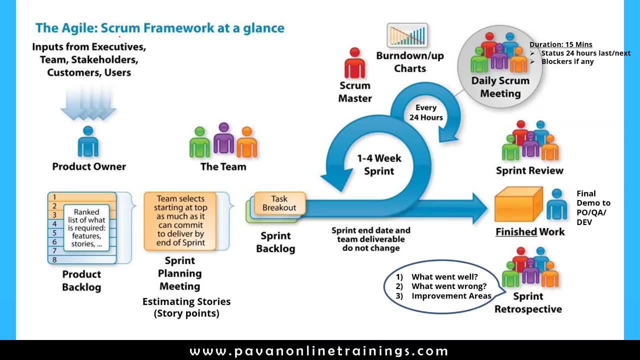 So all these things will be discussed during the sprint planning meeting. Okay, Now let's see the picture, and then we can easily understand this. So agile is nothing but a scrum. here There is another term called a scrum. Scrum is nothing but a team. 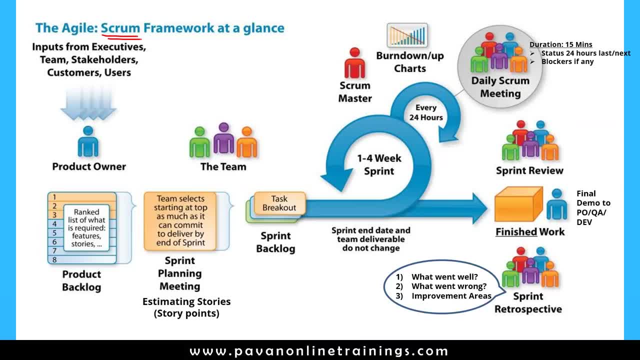 Scrum team is nothing but a scrum master, product owner, developer, QA- So all together we call it a scrum team. Okay, So here the first role starts from the product owner. So what the product owner will do is he will take the input from executives, teams, stakeholders. 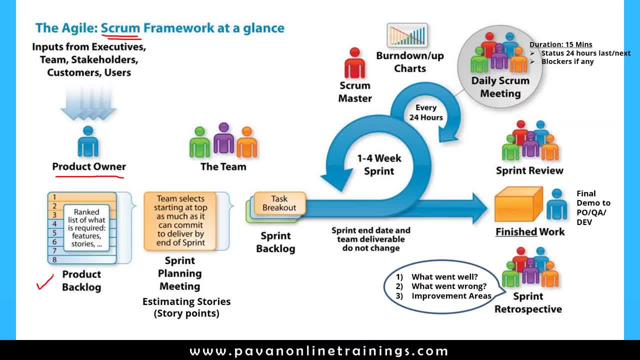 customers and users And he will prepare the product backlog. So what the product backlog contains? the product backlog contains all the requirements, like epics and stories which are given by the customer. So these are first step And once they have the product backlog, so they will plan sprint planning meetings. 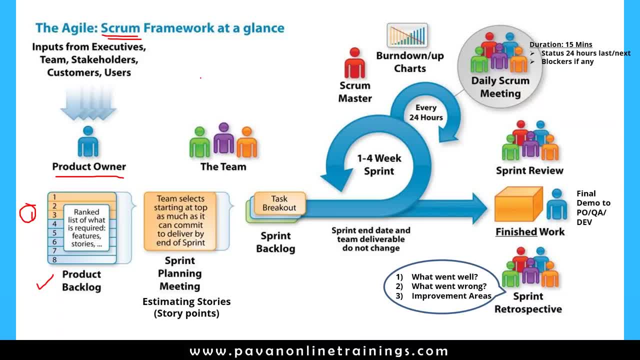 Sprint is nothing but two to three weeks of time. So before sprint is starting, let's say sprint is starting so and so date and so and so it ends. Let us say 1st September it will start and let's say 15th September it will end. 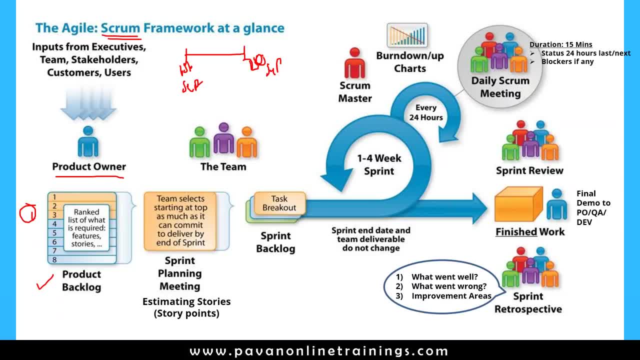 Or 20th September it will end. So almost three weeks of time, So between these sprints. so before starting the sprint time, we need to plan it first of all. Before one day. we have to plan the sprint Now. here it will start. 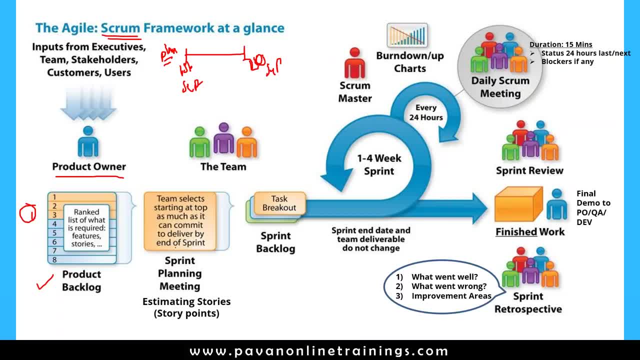 So sprint planning meeting will happen. So what we need to do is sprint planning meeting. So in the sprint planning meeting, so developers will be there as well as QA also will be participated. Now, product owner will show what are all product backlog, what are all stories we have in the. 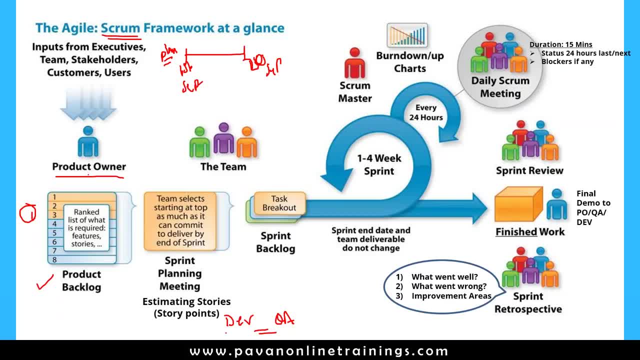 product backlog And develop. and also they. he will say what are the priorities, what are the stories we will need to complete. first, And then developers, and QA means the team. team is nothing but tagging developer as well as QA. So these people will go through each and every story and they will give the estimation point. 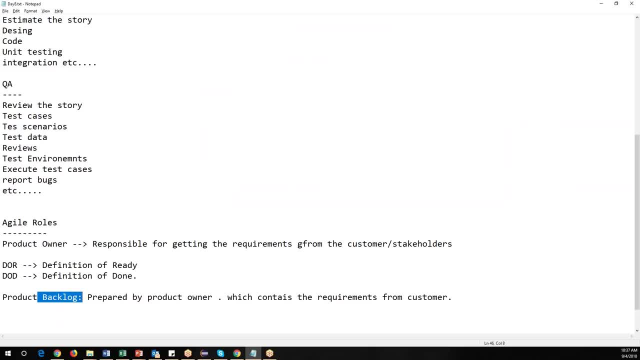 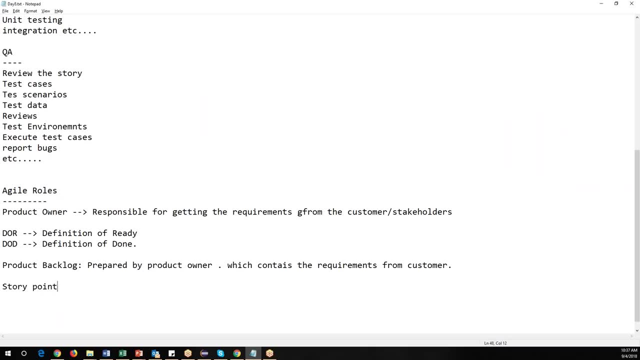 that's called as a story point. So for every story, for every story, there will be estimation point. that is called as a story point. So what is story point here? Story point is an estimation, an estimation even by tester and developer for the specific 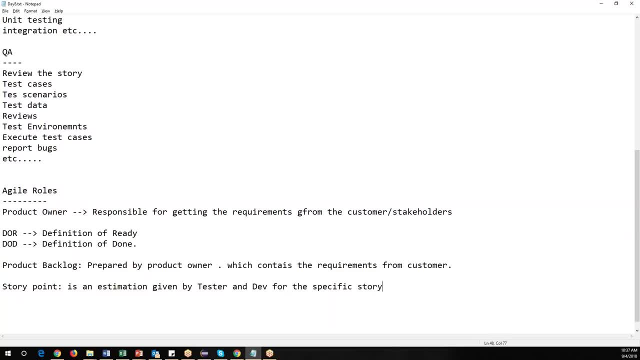 story, specific story, So that is called as a story. point is a kind of an estimation, means a. so I need to decide first: Okay, This is a story, whether it is complex or medium or very small story or not. So for that we need to, uh, I need to. 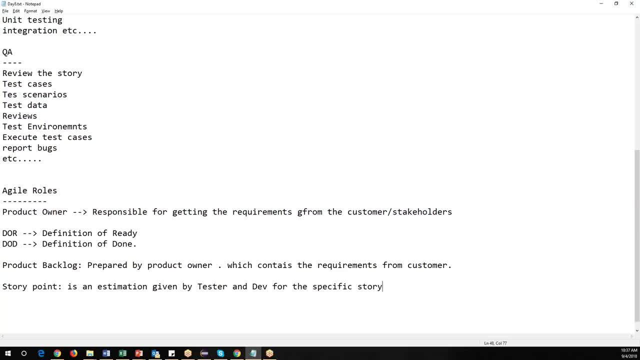 Okay, I need to plan my task. So what are the different tasks I need to do for that particular story and how many, how many hours each task will take? So, based on that, we need to give it a story point. estimation is called as a story point. 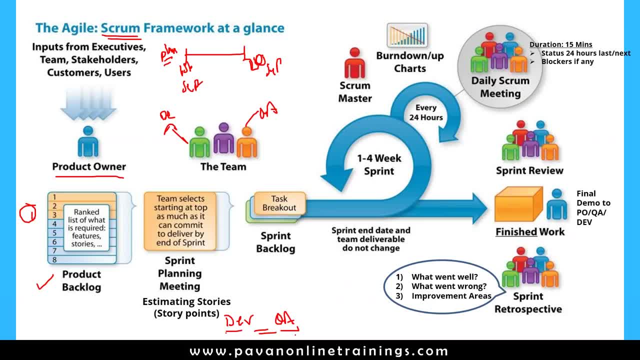 estimation. So during sprint planning, developer as well as QA will sit together and they will give estimation for every story. And normally this estimation will give you in the Fibonacci series, not in the hours, not in the days. Okay, Remember this. Estimation is always gives in the form of a Fibonacci series. let's say here: 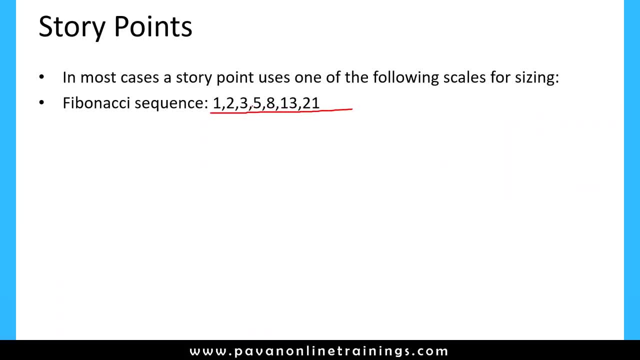 So 1,, 2,, 3,, 5,, 8,, 13,, 20, this is called as a Fibonacci series. So these are not representing number of hours. These are not representing number of days. Okay, Estimation is nothing but the rough, rough one. 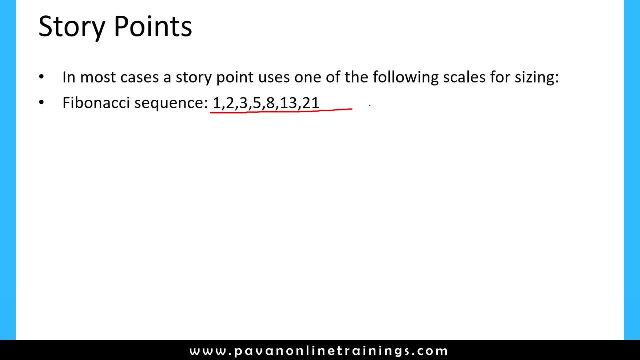 So we are not guarantee like we have completed work. we have to completed work before this time and after this time. So estimation is just a rough estimation, So this is not a hundred percent fixed. But uh suppose if we we have completed work before this time and after this time. 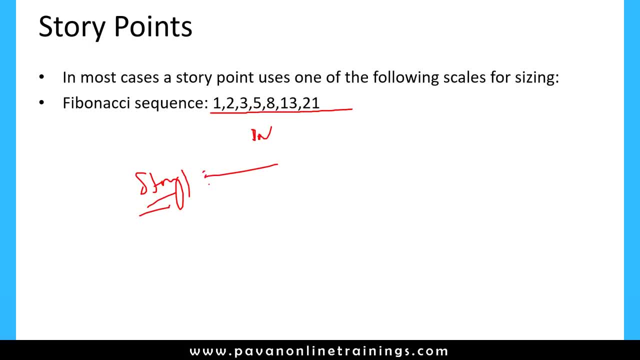 Let's say we have a some story like this, so developer will give you some number to this story. Okay, So this story seems very complex, So I need a lot, of lot, much time and a lot of hours I need to spend. 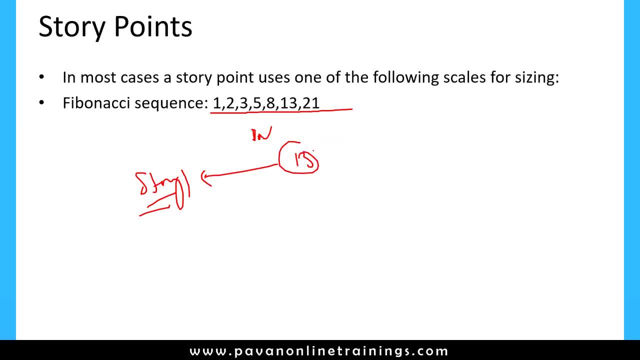 I can just say 13 is my story point. So he will think that and similarly QA point of view, QA guys also will give the same estimation for the same story. and let's say QA activities are different and dev activities are different. Sometimes the developer will take a lot of story points, but sometimes we'll QA take. 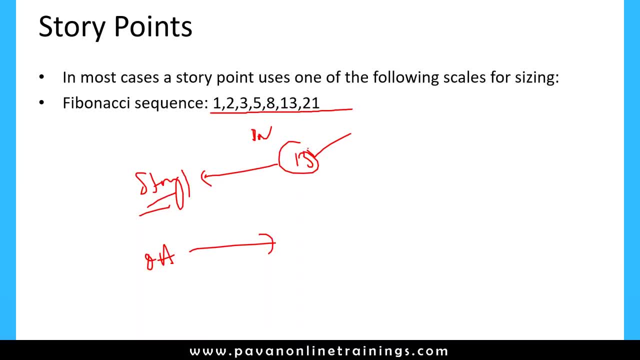 less number of story points And sometimes a developer will may need less number of story point, but QA talks are very high And sometimes QA will give a lot of more story points. Let us say QA people is given story point as a eight and on an average they will take. 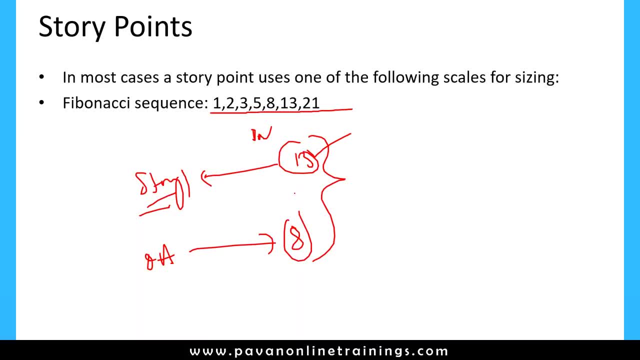 So between eight and 13,. so almost a which one is highest or how many votes they are getting more. Suppose that there are developers are five, you have three, total eight people. How many people are giving 13 more? So how many more people giving 13 or eight, based upon the number of people, based upon 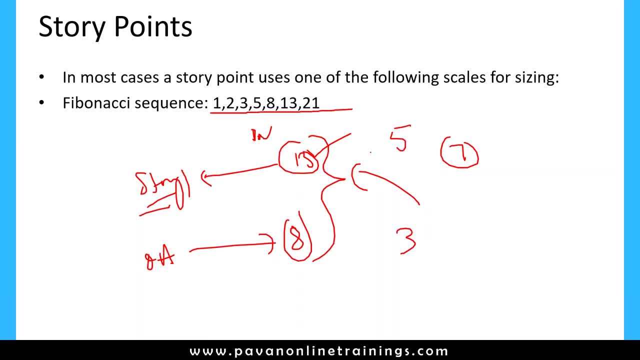 the size. Suppose let's say seven people are giving 13 and the rest of them are giving just eight. Okay, And then they will finalize 13 as a story points. So like this, we have to give a dev as well as QA. both will give you a story point estimation. 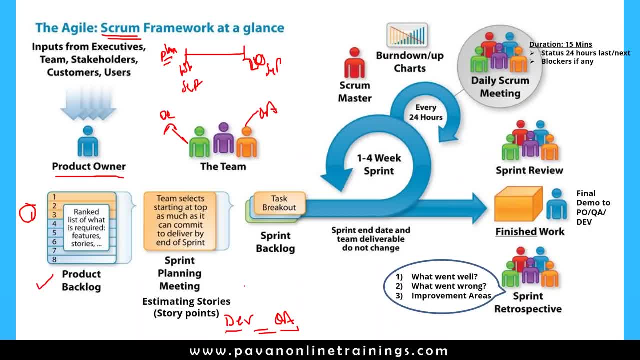 for every story. Okay, Based upon the tasks and, finally, which one they will finalize. So So the maximum voting they will consider. So there are number of QA and number of developer. each and everybody in the team should give the story point. 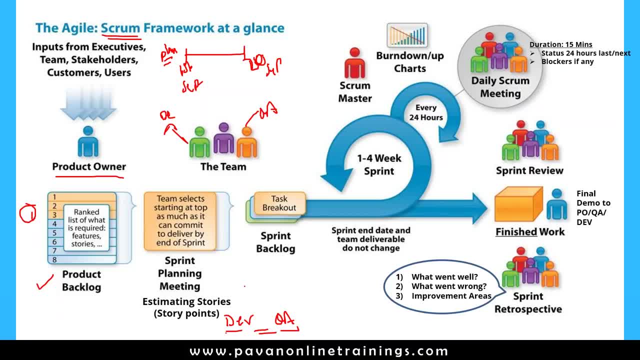 Suppose QA is having five people or two, three people. three people has to give the a story point estimation and developer has five members, or the developer five people should give the story story point estimation and overall it will take the on an average or whoever. 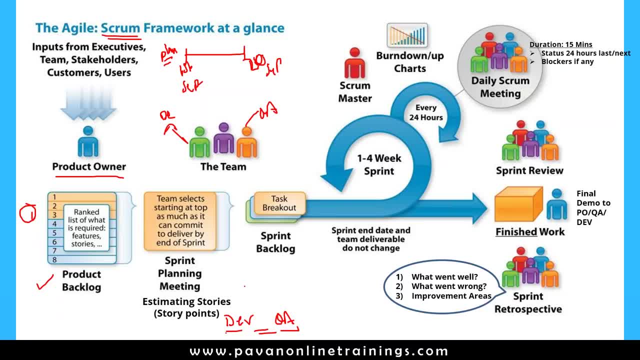 is voting maximum number, So that number will be considered as a estimation story point. Okay, So that thing will happen during sprint planning meeting. So the main activity is one story point estimation, And second thing is they will decide what are all stories we have to implement as part. 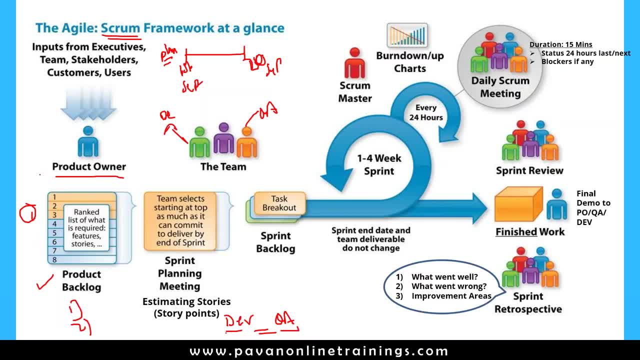 of this particular sprint. So sometimes the product owner says I want to complete, or you guys should complete five different stories in first print itself. So dev and QA will estimate all the five stories and sometimes they say okay, it is possible, or sometimes 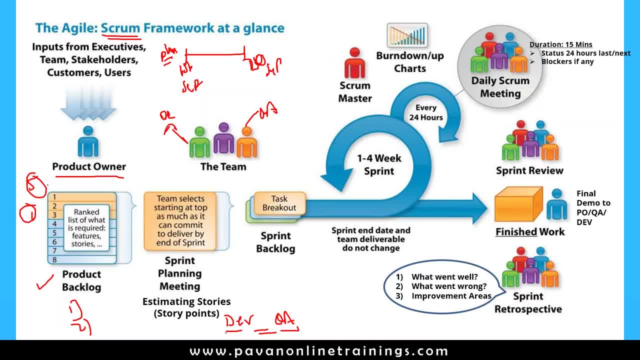 Okay. So if the stories are very complex, then dev and QA will say: okay, we cannot accommodate five stories in the first print itself. we can just implement only three features or three stories in first print and rest of them will implement the next sprint. 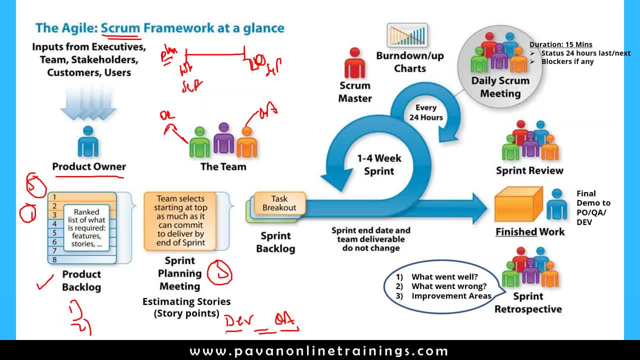 So that's how the communication will happen during sprint planning meeting. Okay, So the product owner will say: always priority, what are the priority prioritizer stories? and, based on that again, developer as well as QA will choose or will commit that those stories. 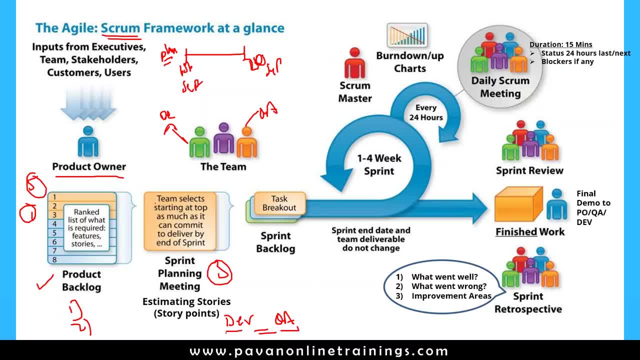 Okay, We were, we are going to develop these stories for this particular spin and testers also will commit. Okay, We are going to test these particular stories in that particular sprint And finally, in this particular planning sprint, planning meeting, they will create one more. 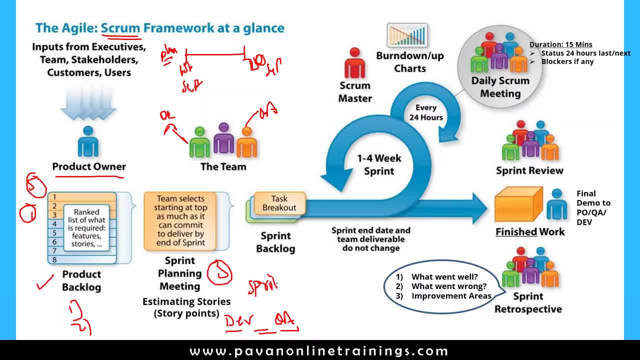 document called as a sprint backlog. This is very important sprint backlog. So now we need to understand the difference between what is product backlog, What is print backlog. So product backlog is a document which will be prepared by the product owner, Which contains the requirement from the customer and stories and epics. 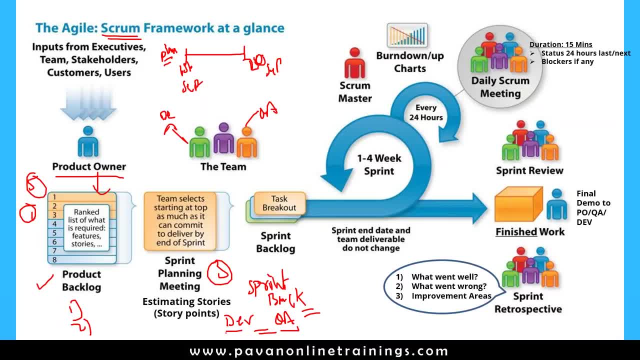 Now in the sprint to planning meeting. okay, we will decide what are all requirements or what are all stories we have to implement and test for that particular sprint. We will commit those requirement. Dev and QA will commit those requirements. So they will list out those requirements or those stories called, as a sprint backlog. 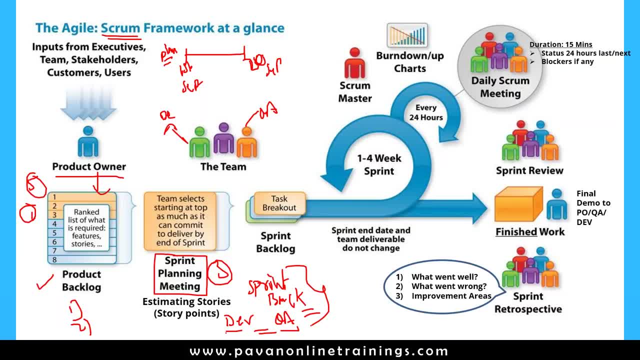 So sprint backlog contains the committed stories. Okay, Sprint backlog contains the committed stories, whereas product backlog contains the complete stories, all the stories which are given by the customer. Okay, So, for example, let us say, in first print, the developers and QA has decided: okay. three. 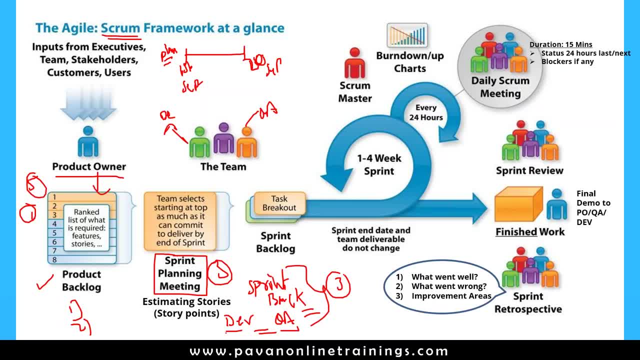 stories we will develop and test, but somehow, because of some challenges and some issues, they were not able to complete these stories. They have, they are able to only complete two stories, But what happens about third story? again, the third story will go back to the backlog. 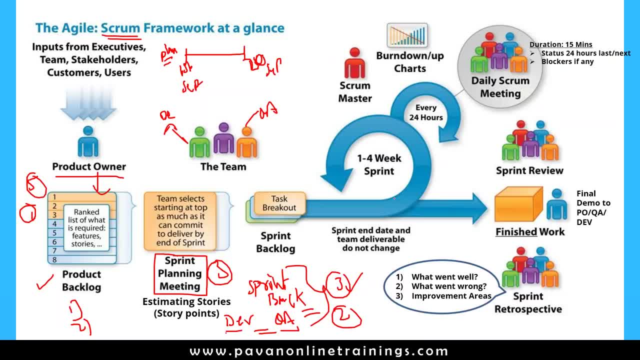 product backlog and they will plan that story in next sprint. Okay, They will plan that particular story in the next sprint, But the developer and QA should justify the reason for that why they are not able to implement this. three, because they have the committed beginning at beginning level. 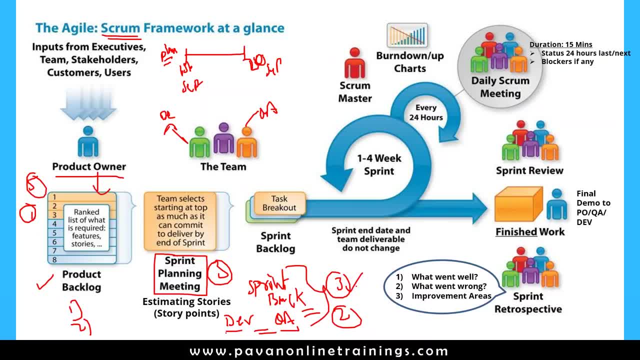 So they have committed to implement and test these requirements, these stories, but at the end of the sprint they were not able to complete three stories. They have completed only two stories. So they have to give proper reason and justification why they are not able to develop these three. 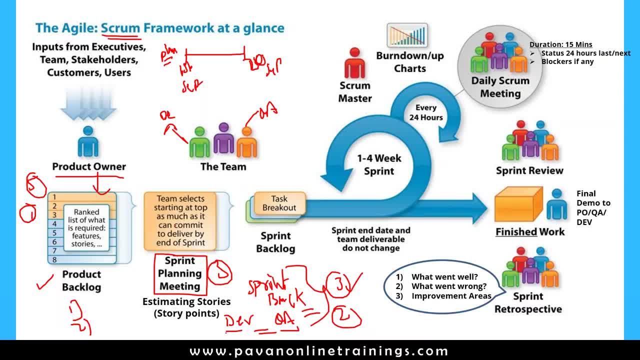 stories. Okay, So that's how the sprint planning will happen. So during sprint planning they will decide what are the other stories they have. They will first estimate those stories and based on the estimation, they will decide what are all stories we can implement and test. both should happen. 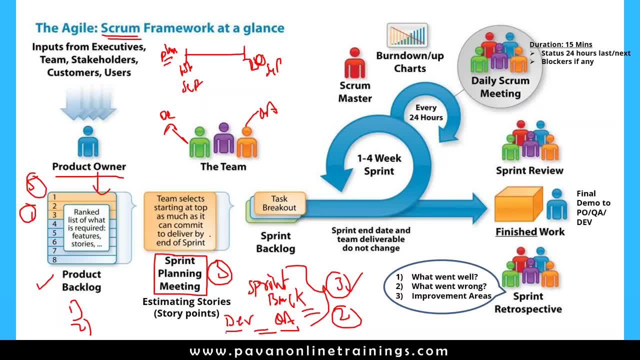 Development, testing, automation. everything should happen within the print itself. So The QA should plan accordingly. So all the tasks should be able to complete for that particular story within the sprint itself. two to three weeks of time. Okay, And they will prepare the sprint backlog. 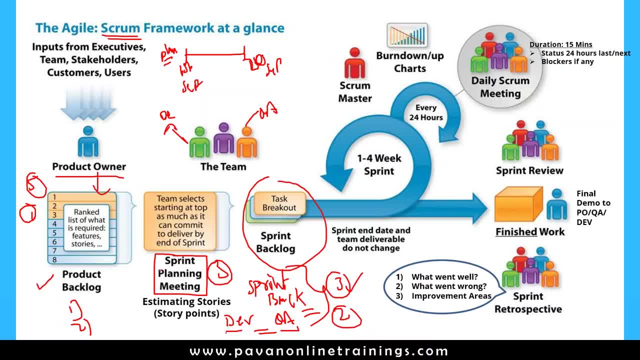 And for each story in the sprint backlog, the developer will write their own task and tester they will write own task. They will define their own task. Normally what the developer task will be: understanding requirements, setting up the environment, creating the unit test cases, develop the programs. 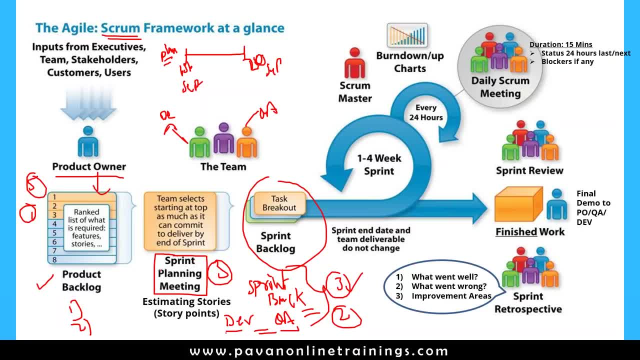 Testing of unit testing or unit testing, integration testing, build creation. So all these things are comes under the developer task or developer activities for that particular story. And what are the tester task for that particular story? He has to understand the story, He has to prepare the test data. 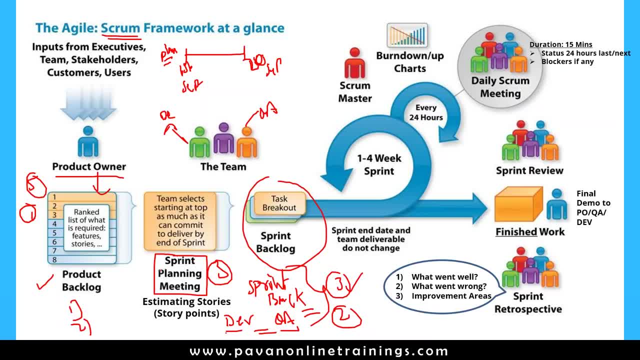 He has to prepare the test scenarios, test cases and making test environment ready- Okay. And build a deployment execution, functional testing, retesting, bug reporting- Okay. All these things comes under the tester task. So, for every story Developer will define their own task and a tester will define their own task. 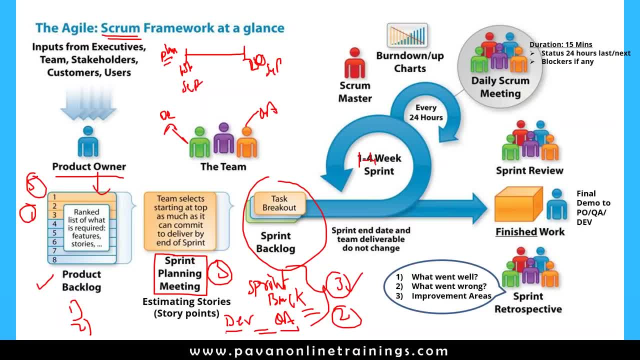 And during this particular thing, let's say one to four week, as I said. right, but not more than one to four means almost one month, But normally the sprint duration will be one to three weeks, not more than three weeks. Okay. 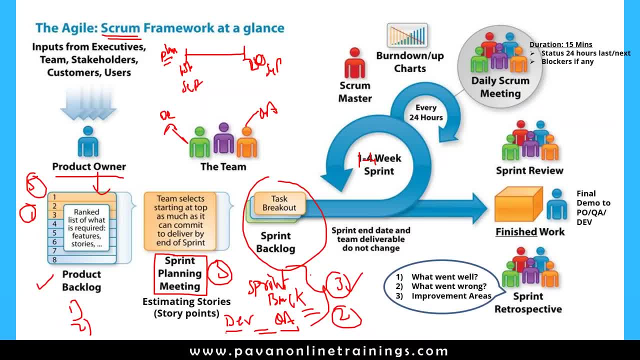 So during the sprint time, so developers and testers will work on that particular story And within the sprint itself, all the testers and all the developers should complete their tasks. Okay, And they have to complete this task And once they have completed their stories, they have to give demo to the stakeholders. 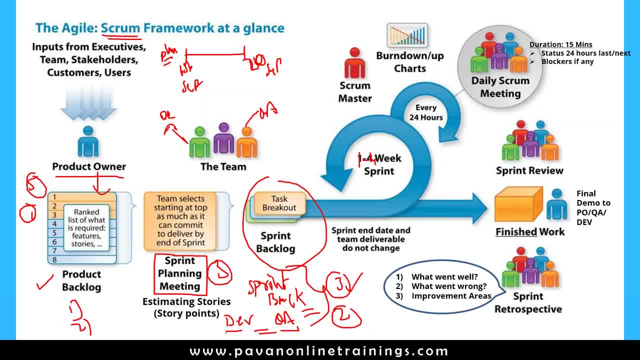 or product owner, QA dev, everybody, And before that, this particular sprint cycle, scrum master will organize everything. Okay, Scrum master will be very important role during the agile process, So he will monitor the complete process how it is going on. 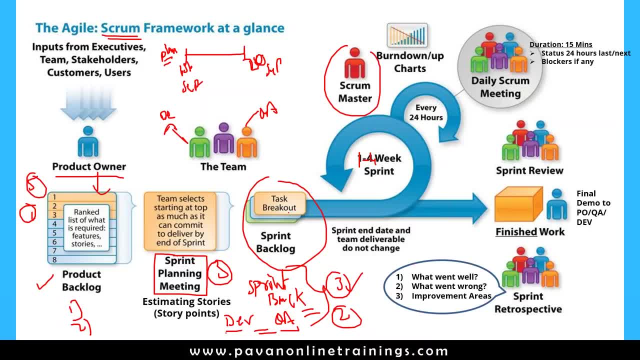 So what are the stories? Okay, The stories they have committed. So how the progress is going on, or dev, or QA said any challenges they are facing or any blockers are there, how to resolve them. So are we good to go or not? 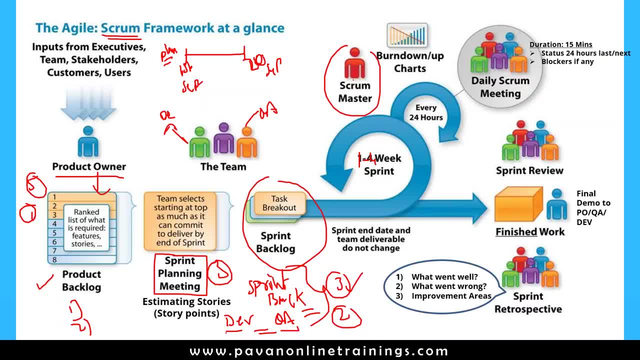 So any blocker, so all these things are taken care of by the scrum master. So he will monitor the complete status of the stories And here within the two to three weeks of time, the sprint will going on. So during the sprint, every 24 hours- that means every day- there is a meeting called. 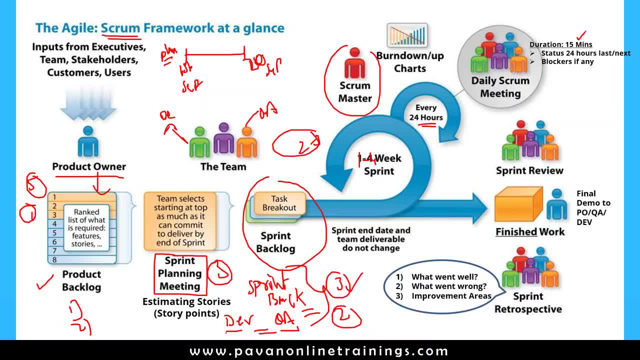 15 minutes of meeting Every day. we have to meet within 15 minutes. everybody will be part of that particular meeting, So that's called as a scrum meeting. Okay, This is called as a daily scrum meeting. every day, 15 minutes. the meeting will be happen. 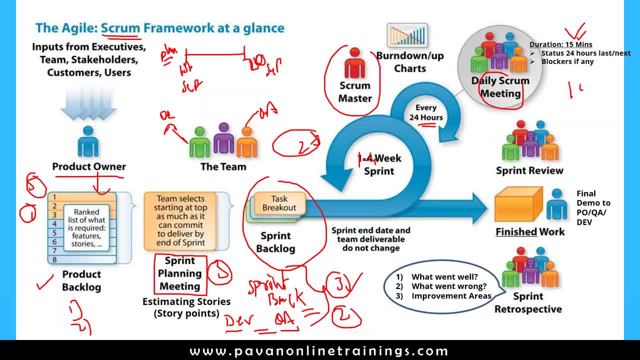 and over is part of that particular scrum. Let us say 10 people are part of that particular team and each individual should give their status. Okay, So in that particular status what they will think they don't discuss more things, Okay. 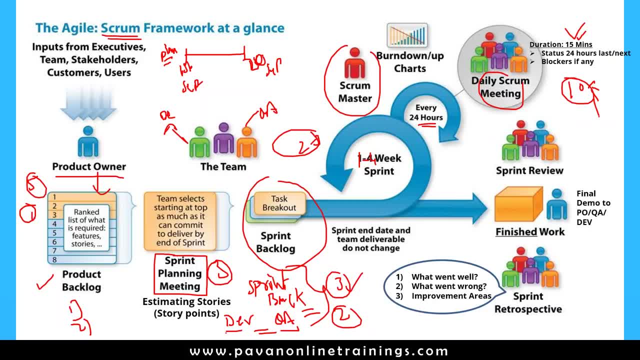 They will just discuss about the progress, not other other things. only 15 minutes, So here they will just discuss about what is the status from the last 24 hours, what we have done last 24 hours and in the next 24 hours, what you are going to do, what is. 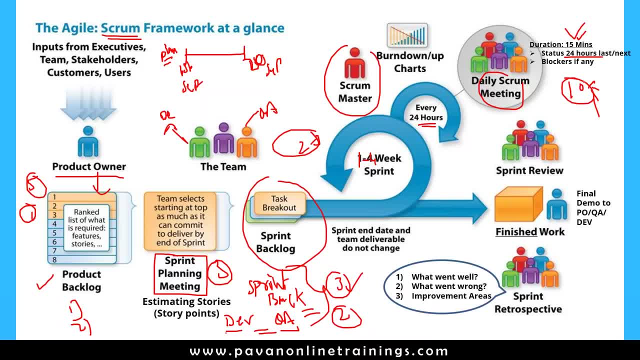 your plan And if you have any blockers or not. in the last 24 hours you have committed to do. you have already committed to do something, but you have not completed. why it is not completed? Do you face any challenges or not? Okay, 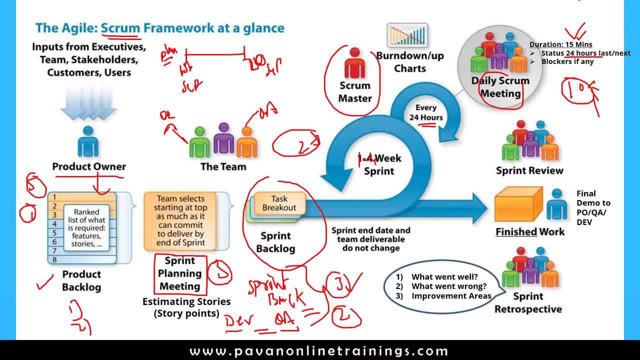 Do you face any challenges or do you have any blockers? So those things we have to discuss during this particular meeting and in this meeting, developers and QA and scrum master- sometimes the product owner is also part of this meeting. So every day, 15 minutes of time will spend to discuss the status of your stories. how. 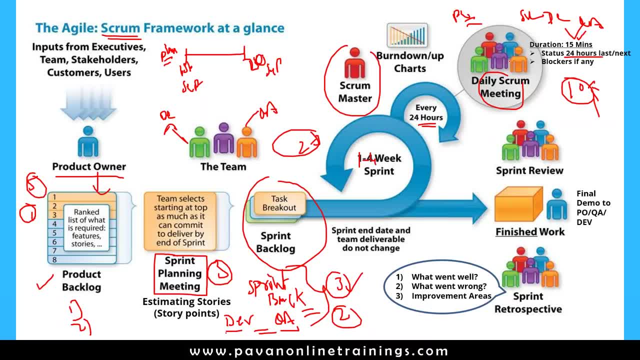 they are developing developer is doing, how the testers are doing, how the developer tasks are going on time or not, and the tester tasks are going on time or not if they are facing any issues. So all these things will be discussed during this scrum meeting is called daily scrum meeting. 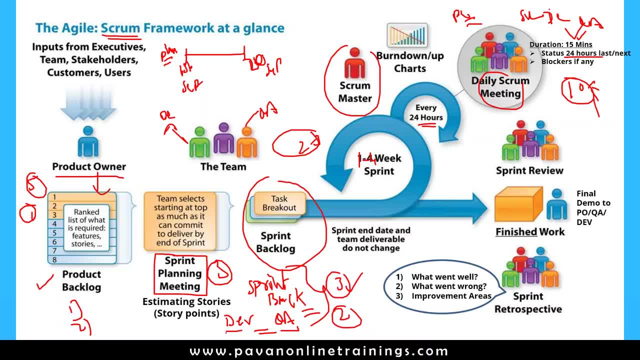 So every day will happen during the span of pre-sprint, Okay. So once this is completed- okay, two to three weeks sprint is completed. So one version of the software is ready. So we have developed this story and we have tested the story. 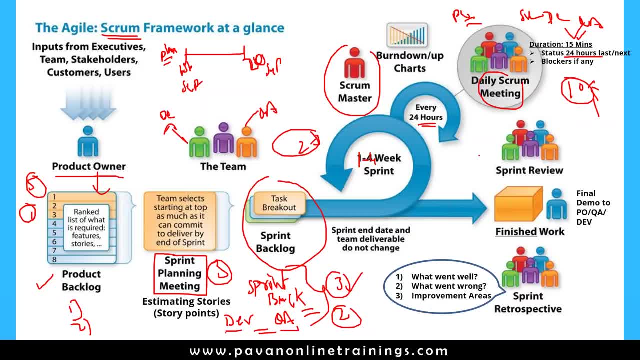 Now, before releasing to the customer, we have to give the demo to the all stakeholders means especially about: product owner should approve the demo. Product owner should talk to it. Okay, So here, once the completed this, we need to give final demo to product owner QA team. 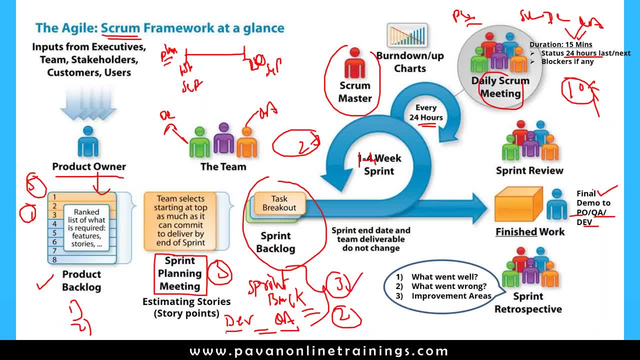 as well as demo. So normally these demos are given by QA people because they are the testers, right? So once they have done the testing- complete stuff- they will set up an environment and give the demo on the story- how it is working- to the product owner. 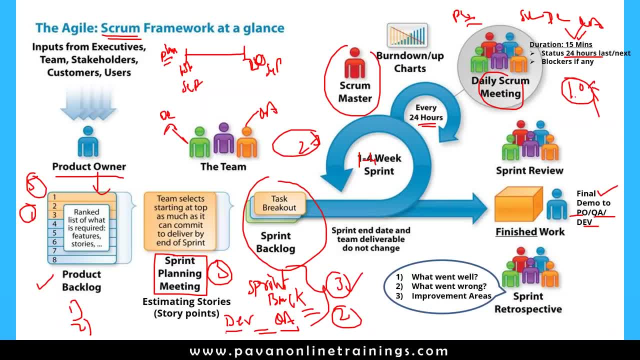 Product owner doesn't know how the developer is implemented, how the testing is done. So ultimately, what he will say is: what is the customer requirement, Whether or not it's a product owner, Okay, Whether my product is working to according to customer requirements are saying or not. 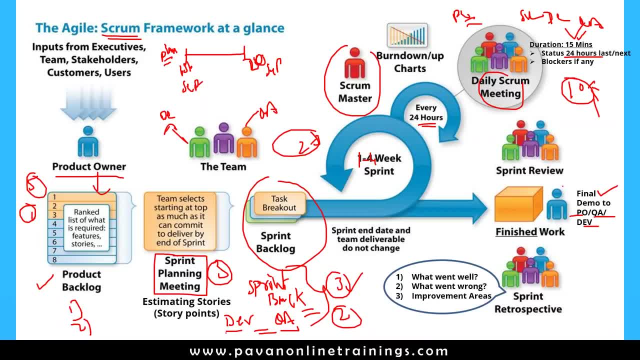 So the only the taking care by the product owner. suppose if the product owner doesn't like the design or development and outcome, again he can reject our development and testing. So again we need to start from the scratch. Okay, So develop a product owner is a main responsible person. 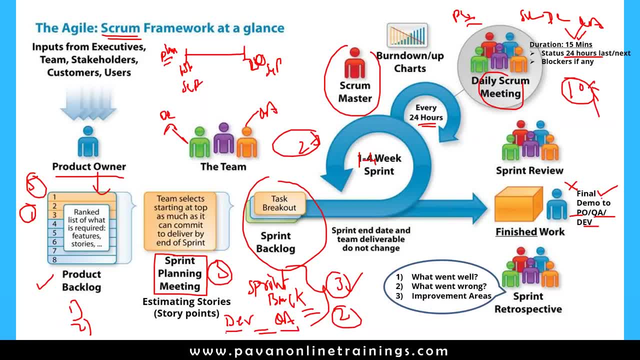 He has to give us a requirement and he has to approve the product. Okay, So after completion of the sprint, we finish that work and then we'll give the final demo to product owner QA as a dev and we'll finish the sprint. So this is complete the sprint life cycle. 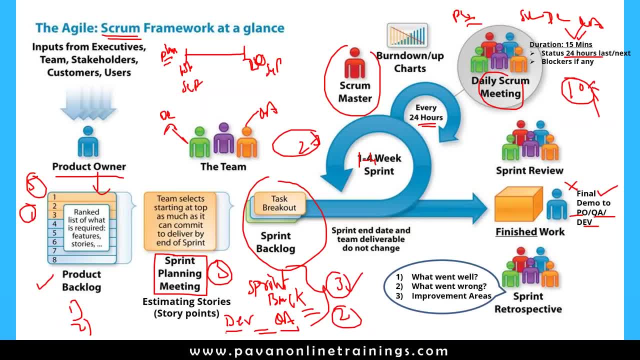 From the product backlog. we'll have the sprint planning meeting. During that meeting we will estimate the story points, We'll choose the stories to develop and test, in particular sprint, And during two to two weeks here, a developer will design their tasks, QA will design their. 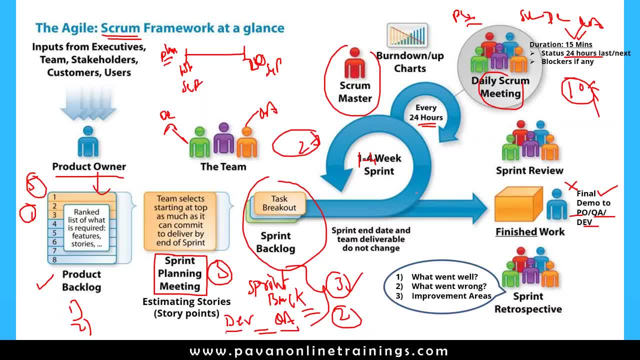 tasks. They will complete their tasks within the two to three weeks of sprint And finally, once the story is completed, they will give the demo to the product owner. They will give the demo to the PO, QA and developer team, and then sprint is completed. 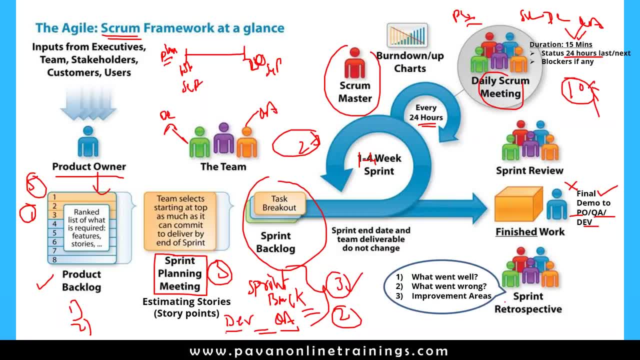 So once the sprint is completed, at the end we need to do set an meeting here. Sprinter is a retrospective meeting. This is the last meeting we have to conduct after completion of the sprint. So what is this meeting is in this meeting, all the team people meet together and they 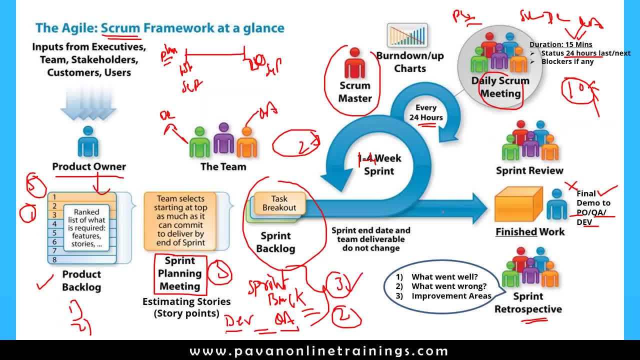 will discuss in that particular sprint, during the sprint, what we have done well. So What are the things that went well? and what went wrong means what are the challenges we face, Okay, Why we have delayed some tasks and why we are not able to complete the task on particular. 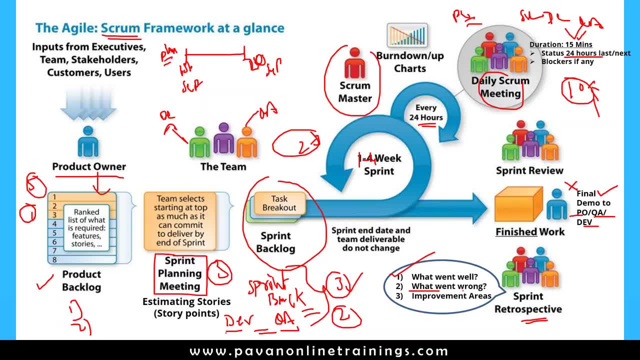 time or committed time. So those things we will discuss. what went wrong and what are the improvement areas we have to do for the next sprint, So those things will be discussed here. This is called as a sprint retrospective meeting and this meeting will be conducted after completion. 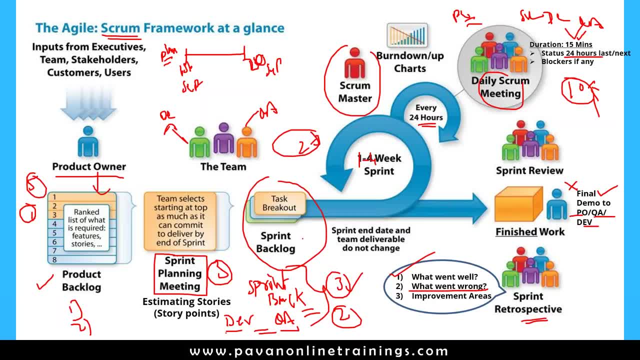 of the first sprint And like this, there are multiple sprints. We will go on till we release the complete product to the customer. So multiple sprints will be going on till the release time or release deadline, and every sprint, the process is same. 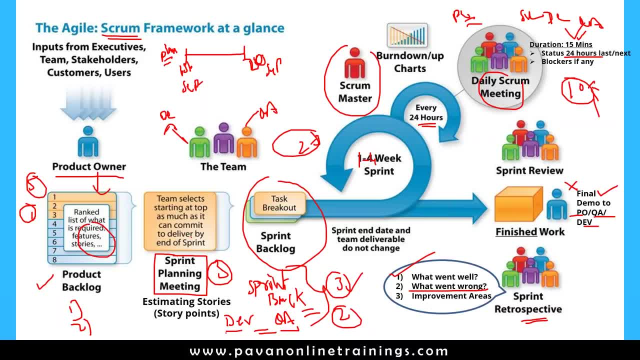 So again we will take few more stories and again Dev and Q will estimate those stories, again plan it or committed those stories for the sprint to again in sprint to also developers and testers will design their tasks and complete their tasks and give the demo, and every day 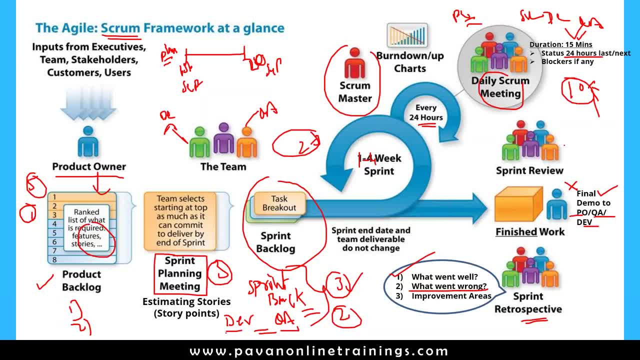 they will have some meeting to discuss the status, So all these things will go as usual. Okay, and this is how the agile process will work. So the main we need to understand is roles: product owner will prepare the product backlog, and developer and QA will committed the stories which is part of sprint backlog and these 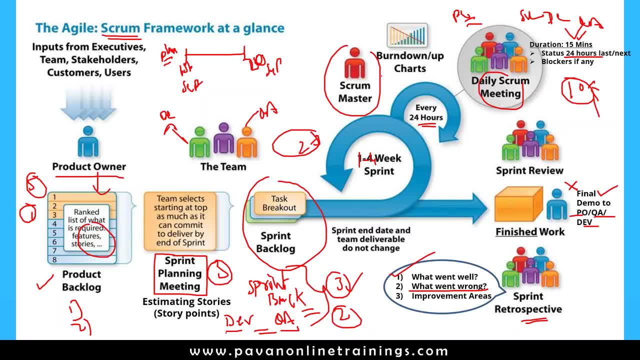 stories will be done by the developer and QA scrum master is a guy who is managing the complete agile process. Okay, so, if there are any challenges, if there is processing is delay, or if any blockers, he is the responsible guy to talk to the management and and finally, he will review. 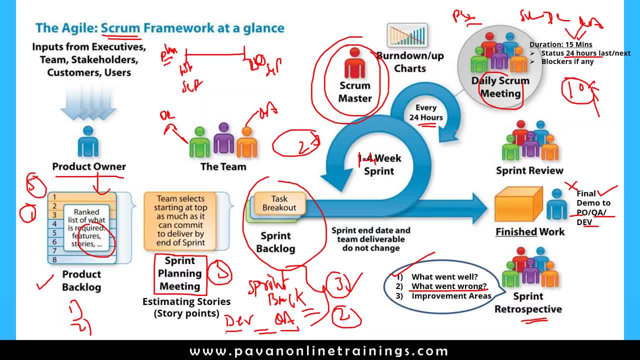 So, like once the Sprint is completed, they need some metrics like how much we have put, how much estimation we have done before and after completion of the Sprint. did we achieved correctly or did we done the correct estimation or something more time we have taken or we? 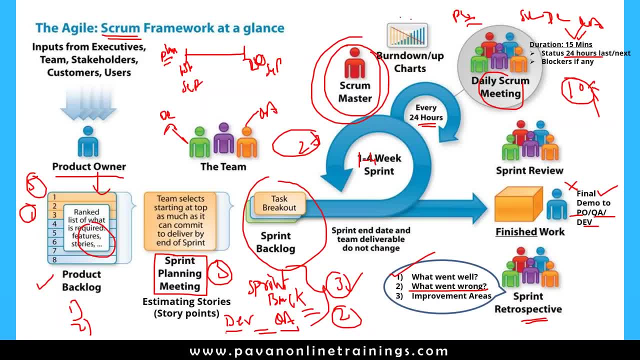 have completed within the last time. So how they will know? so by using this charts burn down and their velocity charts. There are some metrics we have. so, based on the metrics, They will analyze the process: how strengthen the particular process, go out what is went. 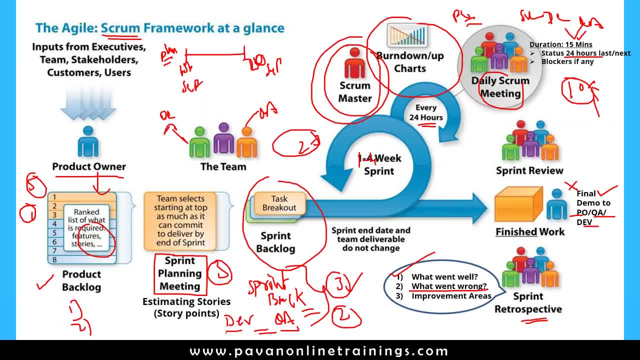 well, and what are the mistakes we have done, how much time we are lacking? So how planning we have done? So all these things they will know about by reviewing the metrics in the form of graphs. So that is again responsibility of the scrum master and program managers and not okay. 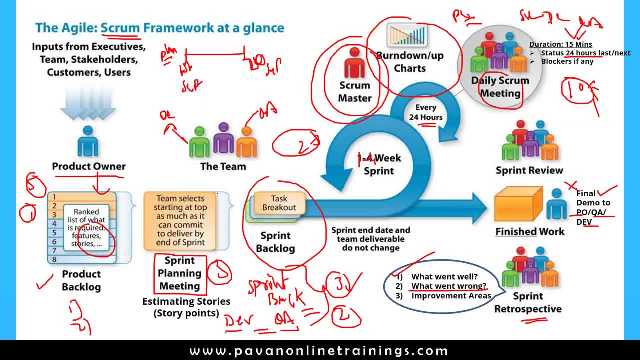 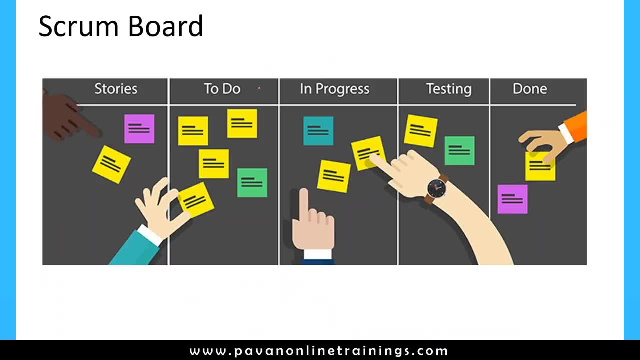 So this is how the complete agile process end to end process. Okay, Now here the main important thing is story points estimation We talked about and this is called as a scrum board. So suppose, let us say, one story, we have, so one story, we have multiple tasks. 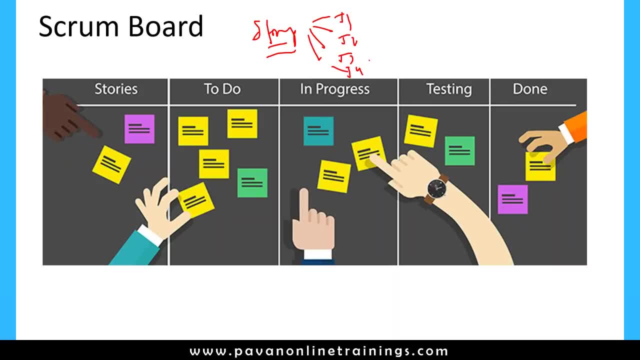 Let's say task 1, task 2, task 3 and task 4, right, So all these tasks we need to, okay. So these are, let's say, story 1, story 2, story 3 and 4.. So this is, this is called as a scrum board. normally scrum master will monitor this particular. 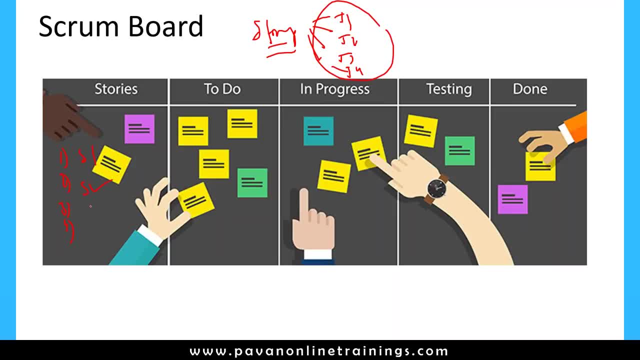 one. So every day we need to tell, let's say, the story 1 here, story 2 here, story 3 here. So this particular story, in which status, your to-do status- or it is in progress, or it is testing, or it is done- it will need to move from space to another sense. 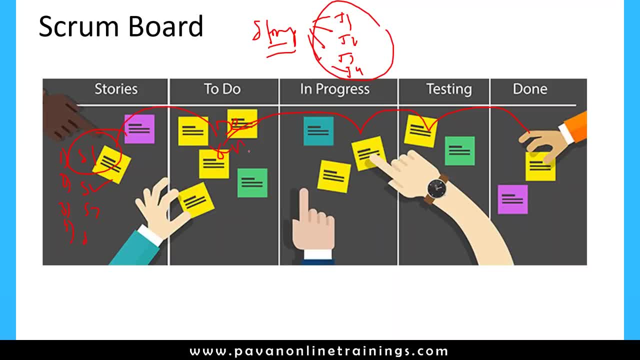 So here to do means again, the developer task will be there, your task will be there and some developer task will be in progress and your task will be in progress and testing during testing phase it is, and then, once the testing is completed, and the story will be. 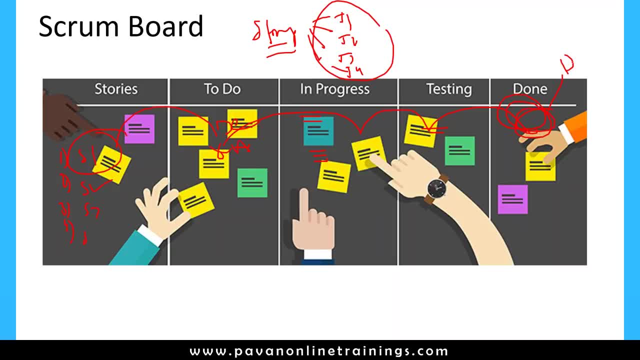 done So once the story is reached till here. this is a demo-able product, so we can just demo to this product owner and stakeholders. So this is called as a scrum board. it will clearly says what is the status of the story. Okay, so to do means it is ready to do, or it is in progress, or it is in testing phase, or 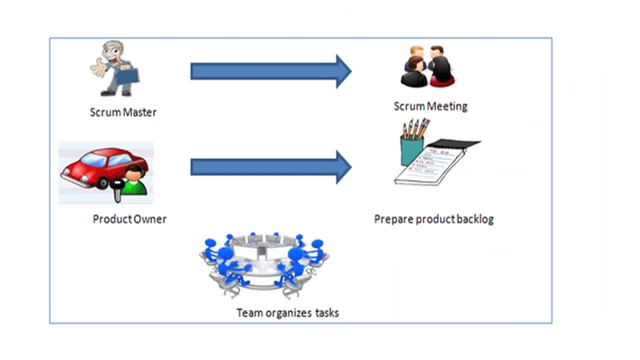 it is done okay. and here scrum master is a role. always he will conduct the scrum meeting with the complete team and he will understand and challenges blockers. if there are any issues, he has the complete team, He has. the guy has to resolve those issues. 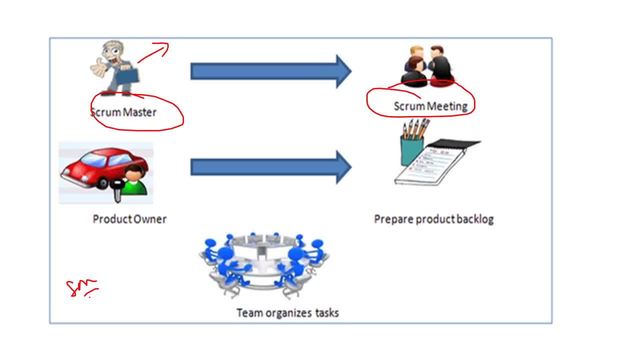 Okay, suppose tomorrow, let's say. in scrum meeting I told, okay, I have some tasks I should able to complete by tomorrow, and again tomorrow I have attend the same scrum meeting. I told, okay, I have planned this task from the last 24 hours but I could not complete that because 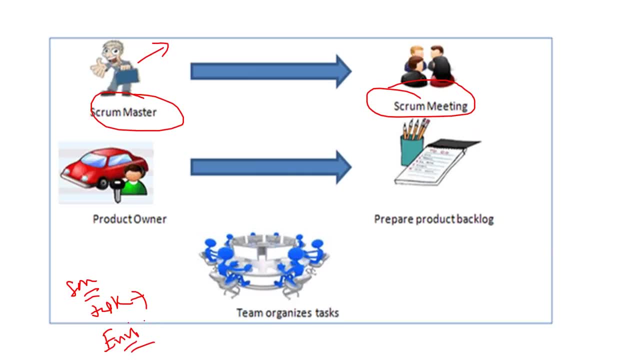 the environment is not ready and I have requested some ticket. it is still not solved. So these kind of reasons and justification we have to do, and then scrum master will follow this one Why it is taking a long time to fix that issue or why it is taking environment setup is taking. 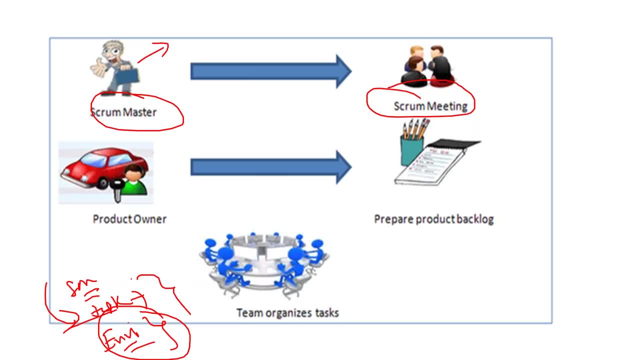 a lot of time. So all these things will bother. we don't bother about anything. only thing is: if you completed our task, we have to just say completed. if you are not completed task on time, we have to say just some small reason for justification and we need to give us a proper reason here. 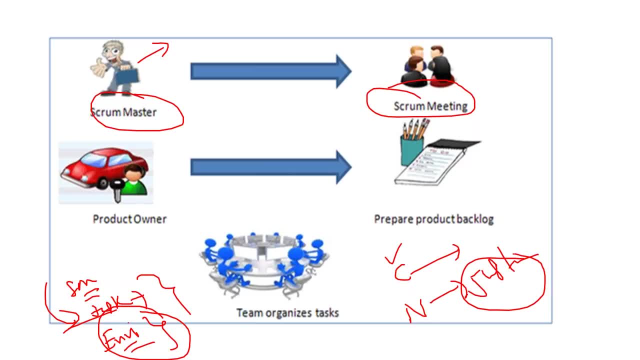 So why the task is delayed? okay, well, if the task is delayed, what are the issues we face, or what are the challenges we face? Sometime we will estimate only something. Okay, So let's say we have six hours of work, suppose in between the environment is not available. 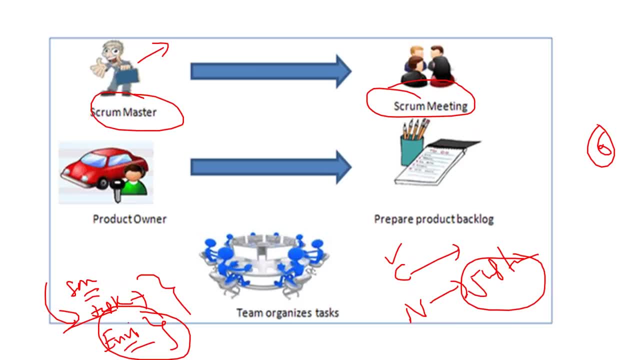 or something is not working properly, and sometimes testing the same scenario will take a lot of time. So it may be extend to a six to eight hours. So these things we need to just justify to the scrum master. So scrum master is a role, is complete, manage the process and product owner is the guy will. 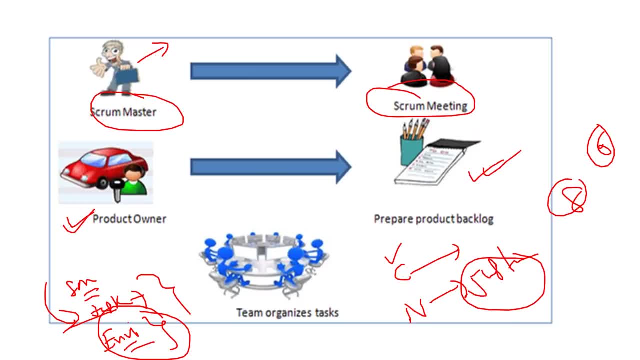 get the requirement and he will prepare the product backlog which contains the all the stories to be developed and test, and team organizes the task. The team is again Dev as well as QA, So these people will organize the tasks. Okay, So this is all about agile process, the complete end-to-end agile process. 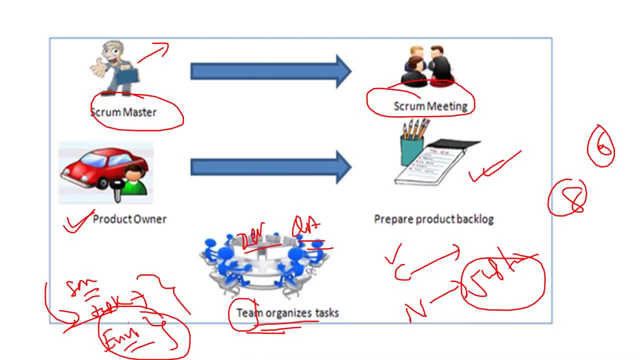 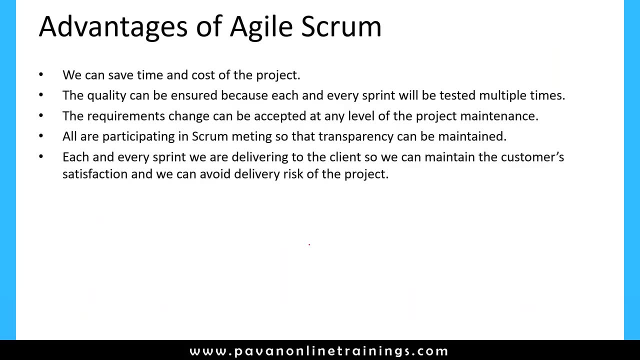 Now nowadays, all the companies are falling that this particular process. all the projects will happen in this particular process. Now what is an advantage of this particular process? So the main advantage of this particular process is customer no need to wait till the last release. So let's say customer is saying 10 requirements. 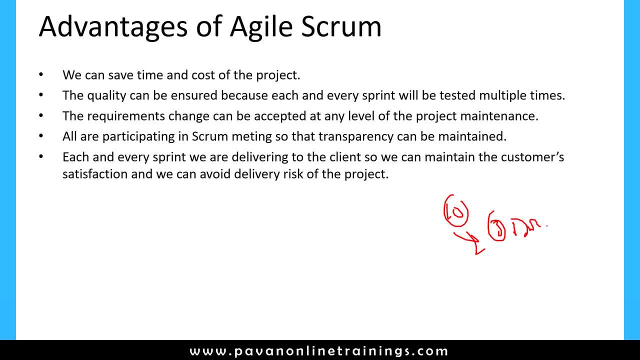 There's a three months of time duration. He should be no need to wait for the three months of time to get the software, because we were developing and testing the software in multiple Sprint. Once we completed Sprint one, he will get the first version of software or, if there, 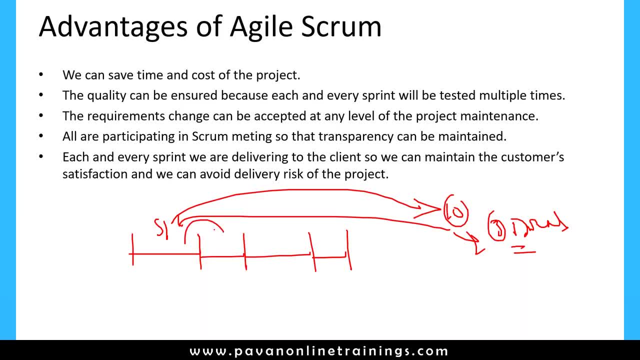 are any changes, you can tell us back and we can accommodate those changes in the next to next to Sprint and we can deliver the next software, next version to the customer. So customer will get releases very frequently. So that's the main advantage of agile and customer point of view. 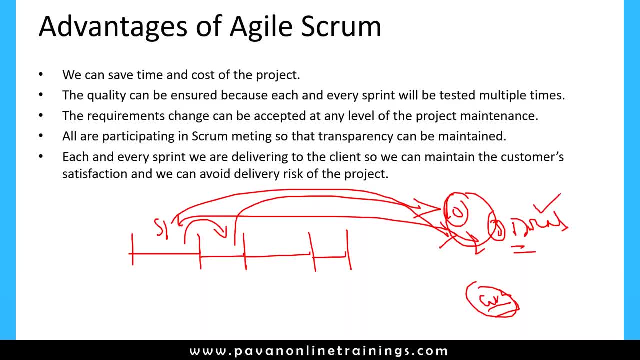 This is very, very useful because you don't need to wait for the long time, and there's a one reason. the second reason is you will get the bills or software in every Sprint and the other other advantages. suppose he want to change something, or if you want to. 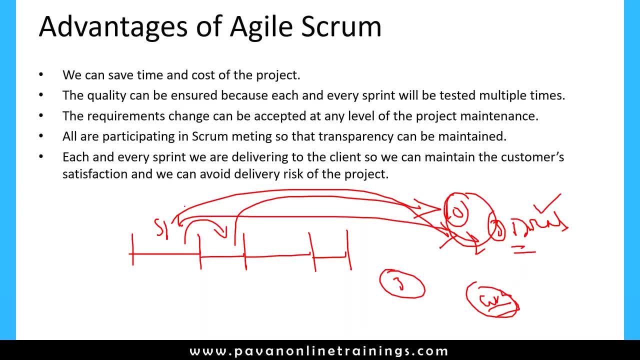 customer. if the customer want to accommodate the new changes, you can immediately communicate with the product owner and then product owner will prioritize that particular story And we can accommodate in the next to print. So there are main advantages of scrum and basically it will save a lot of time and cost. 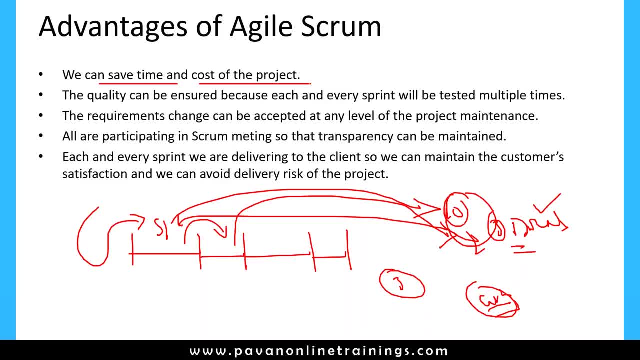 of the project and the releases will happen very faster. releases will happen very faster and they okay. So again, as I said, every Sprint we will deliver a new version of software to the customer. So once the all Sprints have been completed, we will release the complete software to the. 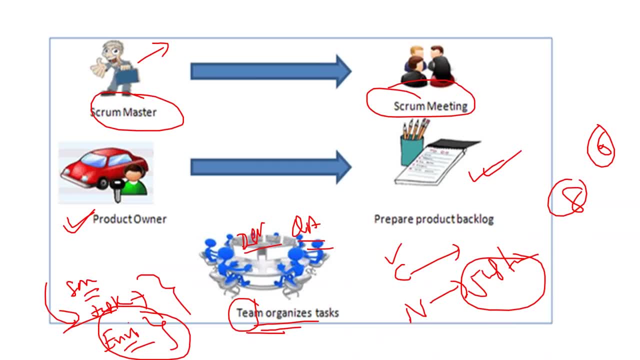 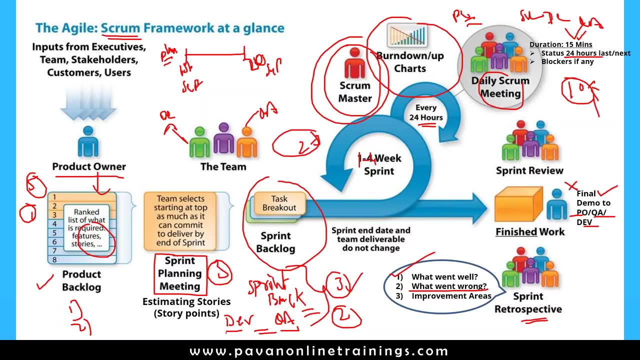 customer. So The agile process will form. So nowadays, every company is using this particular process. every company, almost 90 plus percent of the companies, are using agile process. So any questions so far here on this particular topic, Any questions on this. So now, by using this agile process, we will discuss a small project. 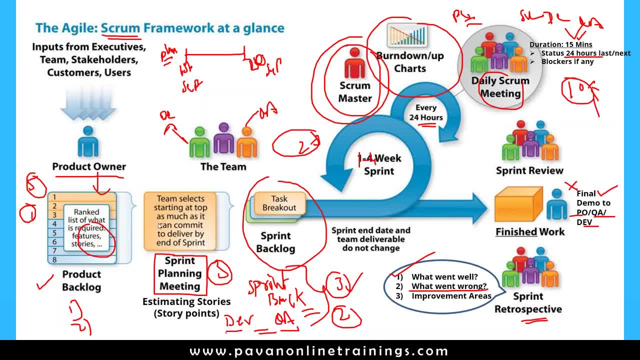 Okay, And how the backlog will be: product backlog and how the Sprint planning or what is the Sprint backlog? how we need to estimate the story points and everything. So let me show you a small document here. So this is a document which is created by the product owner. 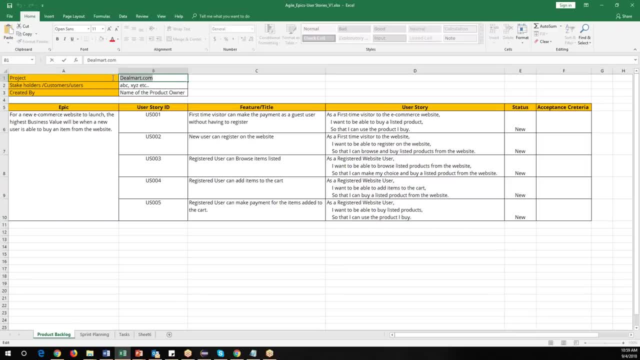 Okay. So here I have taken a small project called deal modcom. It is just like a e-commerce website, Okay, and this is normally prepared by the product owner, not by us, and here they will save over the stakeholders, customers And users here- and they will list out everything and created by the product owner name and. 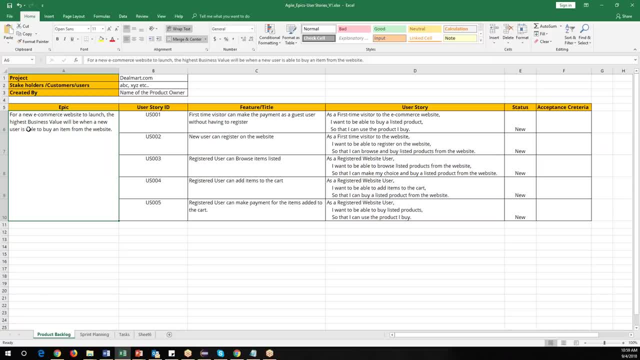 let's say this is our epic. So let's see this an example for a new e-commerce website to launch. the highest business value will be when a new user is able to buy an item from the website. So this is the customer requirement: very high. and for this epic, the product owner is created. 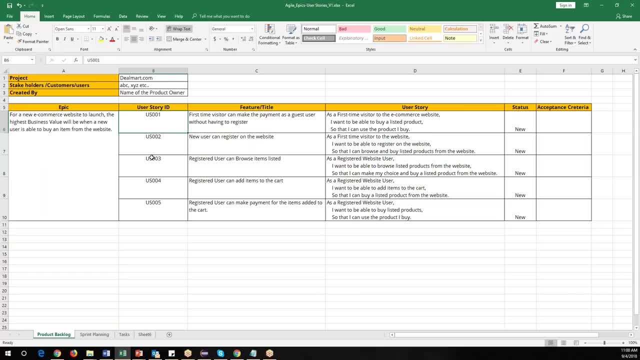 multiple stories, user stories. Let's say they have given us 00100234 and 5. And for every user story they have given some name, feature name or title and say: first time visitor can make the payment as a guest user without having this station. and second, 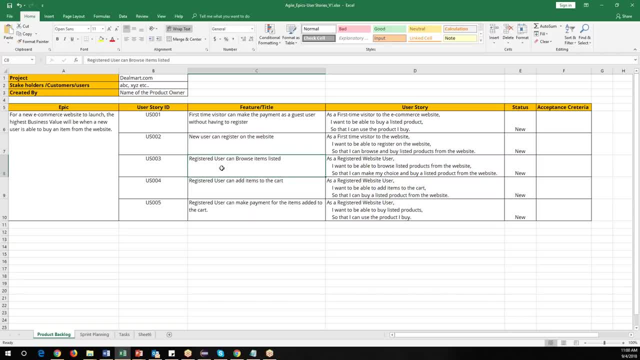 user story user can register on the website and the next story register user can browse items listed and register. user can add items to the cart and register user can make payment for the items added to the cart. So these are the few examples of stories, user stories, and every story is independent and 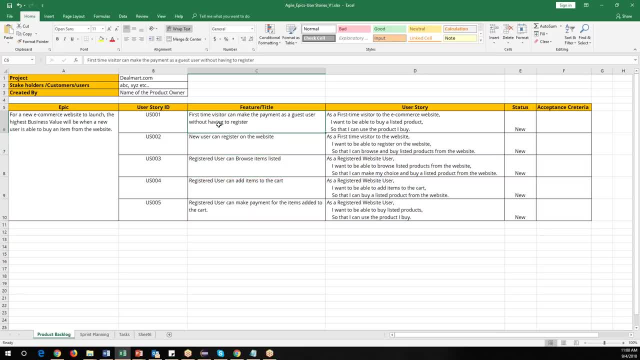 every story will developer will develop and tester will test, and every this is called feature names or title of the story, but this is actual story. So whenever the product owner write some stories, they will follow, set in template or set in format. So if you observe these stories- user stories- almost similar, seems very similar. 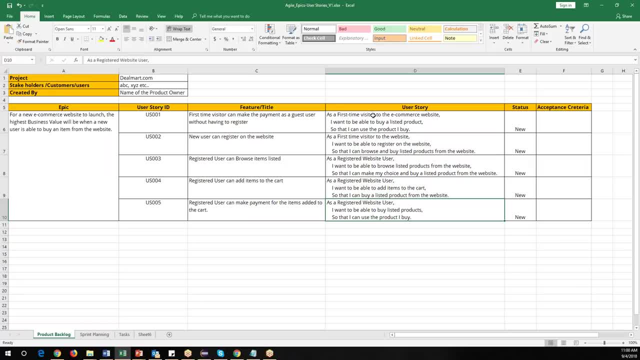 Let's see here They are using some keywords. So, as a first time visitor, So as a first time visitor to the e-commerce website, I want to be able to buy a listed product. Why? so that I can use the product by. so why the first time visitor should able to log. 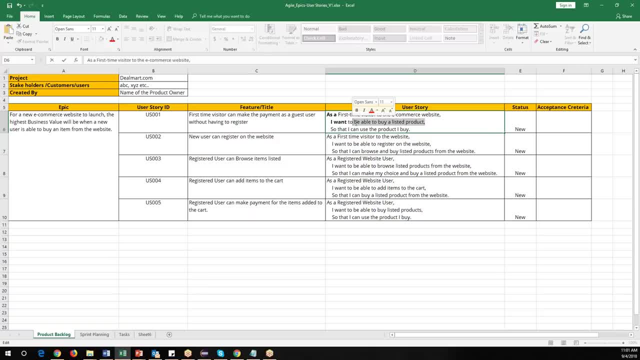 into the website because you want to buy something. and he was to hear: you want to be able to buy a listed product so that I can use the product I buy. So this is a user story. So what we understood based on this is, as a first time visitor to the e-commerce website, 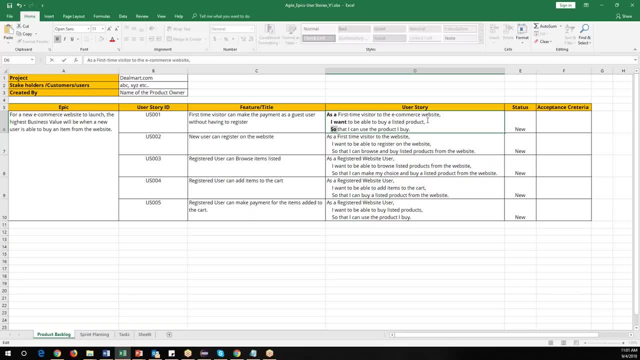 Okay, I want to be able to buy a listed product so that I can buy the product. So before buying the product, we need to list out the product, right? So this is a one story and they are using some common keywords for every story, if you. 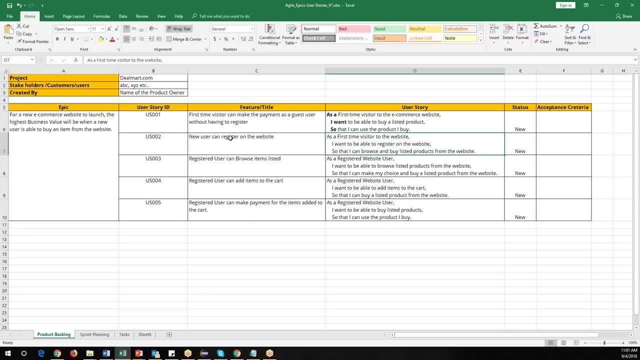 observe here. So let's say second story: So a new user can register on website. This is a feature, and what is the story for this? as a first time visitor? Okay, and to the website. I want to be able to register on the website. 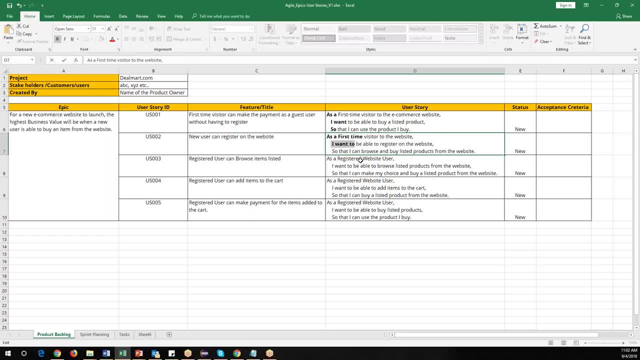 Okay, So that I can browse and buy listed product from the website. Okay, so these are the. this is how we need to write this to user stories. We don't write this user stories. product owner is responsible for writing these user stories, So this is a template they will follow. 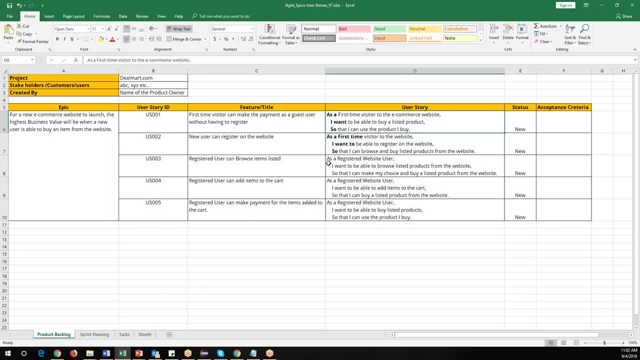 So for every user story they are using this keyword. as a user, I want to do something because I will achieve so and so okay, so we need to do. as a user, I want to do something That represent an action. why they are performing the action? because they are, they want to achieve. 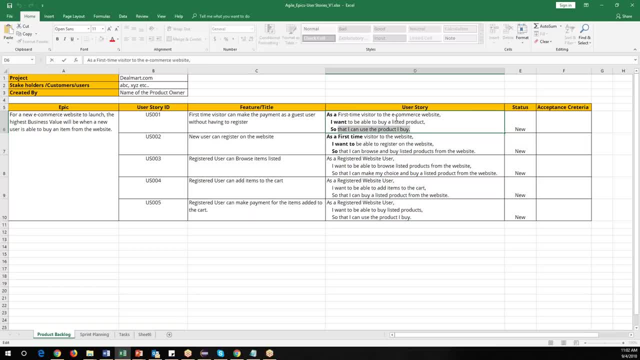 something. So these three should be part of this user story. So user stories describes who is the user, what action he has to do and what is the outcome he will get. So those three should be part of this user story. So when I read the user story, you should get clarity on this. creator. who is the user? 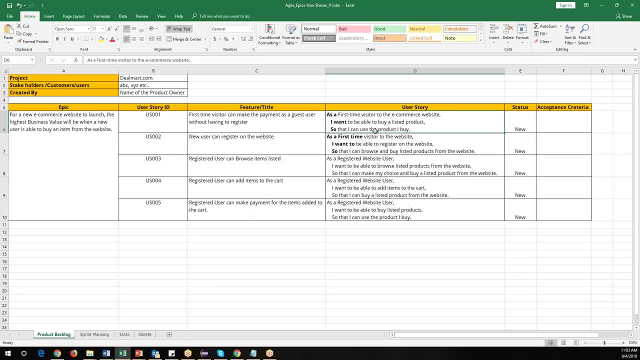 what action he is to perform and what is an outcome he will. he will get out of that action. Okay, So these are all few user stories and they will update the status like it is a new story or it is in progress or it is completed story. these statuses and are updated by the product. 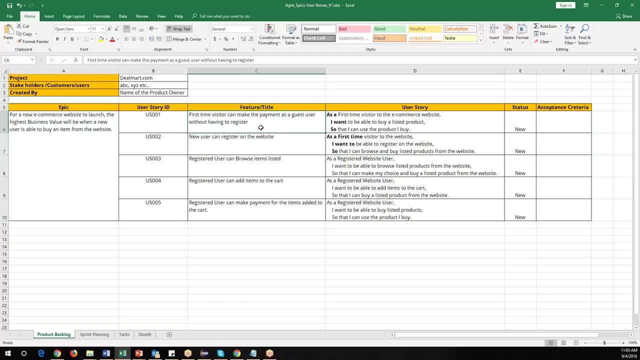 owner later and acceptance criteria? suppose if the story is developed and tested, demo is also done and on what basis the product owner will accept this story. Okay, So if he's accepted the story, he will mention here. what is an acceptance criteria when I need to accept this story? 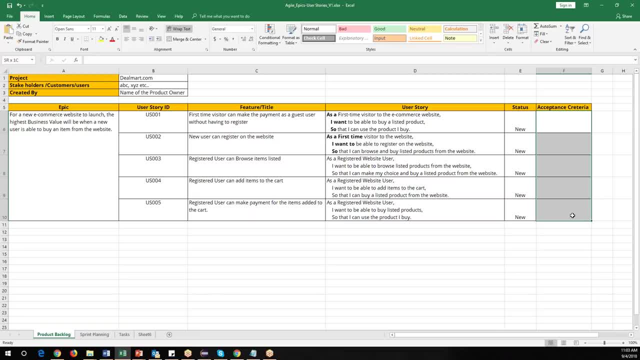 When I need to reject their store. So they will give some certain acceptance criteria in the last corner, and this is also done by the product owner. So we are not responsible for creating this document. So just I'm going to show you is a sample document- how the product backlog will look. 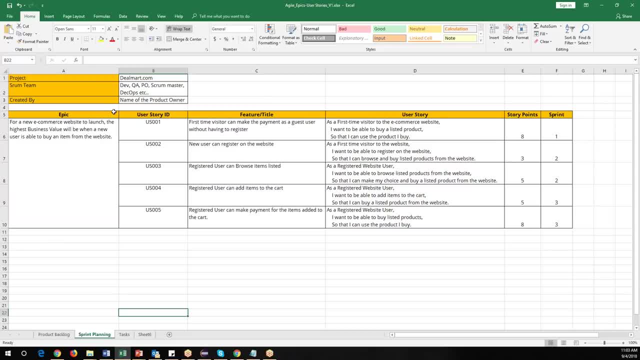 like Okay, and then sprint plan. So in the second stage we are doing sprint to planning. What is print planning? We will estimate the stories and we plan the stories which were developed. particular sprint developer. So, as well as Q activities, we will define: 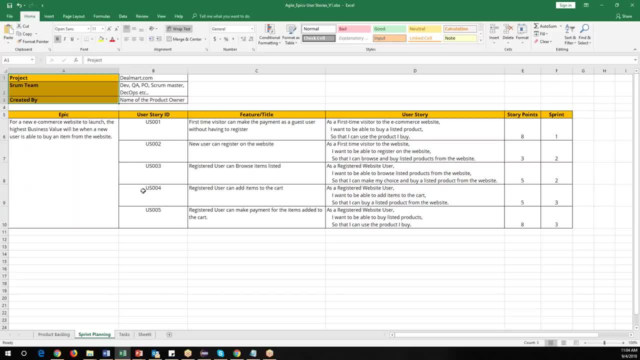 So this is your project name and this is called Sprint backlog. You can say: this is a Sprint backlog, So project name. scrum team, So dev, QA, product owners, scrum master, devops team, So everybody will be part of the scrum team. and who is a creative? so product owner. and. 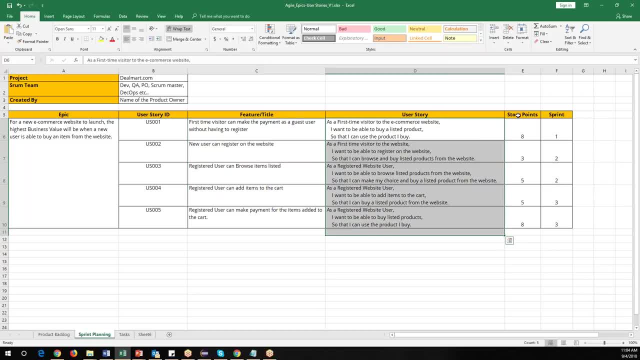 this is a epic and same story, same features, user points. But here additionally, we need to add the use story points and on particular story, on which sprint we have planned. So Let's look on the story points. Let's say it is a complex. these are minimal, size is very less, the complex: it is very less. 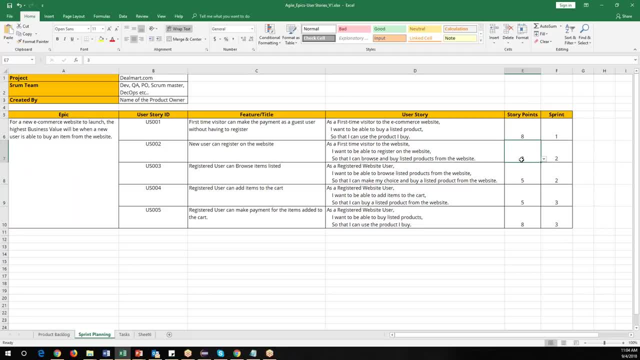 five is medium. five is also medium, So it is a complex. three is a minimum complex and five is a medium. So this is a story points estimation which is decided by the both dev as well as QA. So once we have decided this story points, okay, so they will check the complexity, suppose. 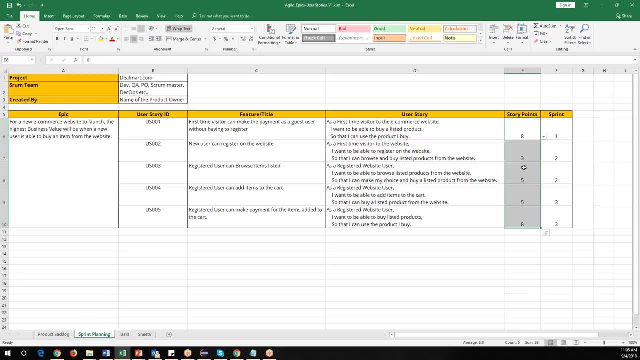 the product owner says: I want to complete three stories in first print. Then developers and QA said: okay, the first two story itself is a eight story points. It is a very complex, so we can complete this. only we can complete this story in one sprint. 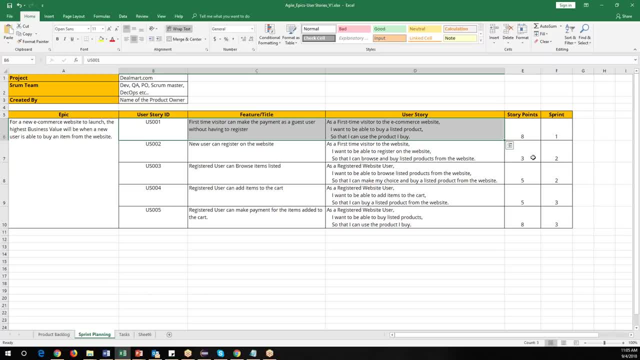 So other stories we can complete in other things. So that is the commitment to the developer and QA should give and so this particular story is planned for one sprint and other rest of the springs are rest of the stories are part of second sprint and other stories are part of the third sprint. 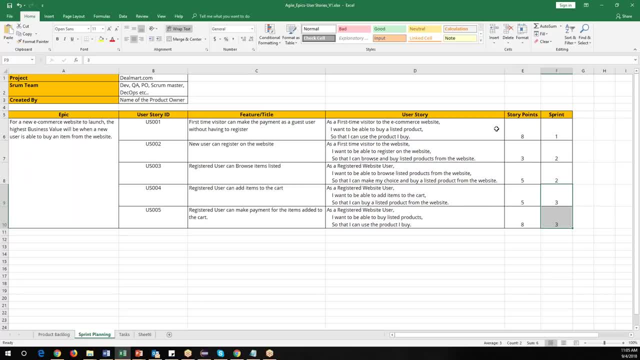 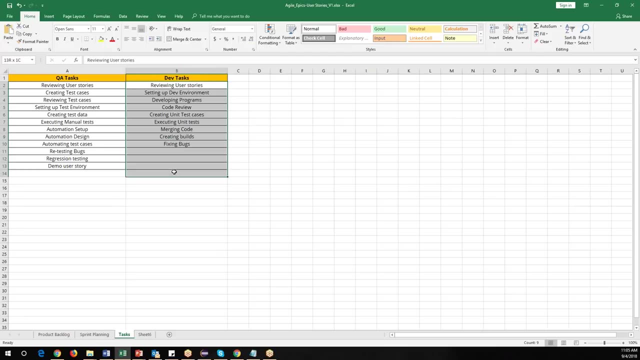 So like this Now sprint planning meeting. so they will give estimation for every story and they will plan that particular story to that particular sprint and for every story. once this sprint planning is done, So for every story, the developer will give you their own tasks and developer QA will. 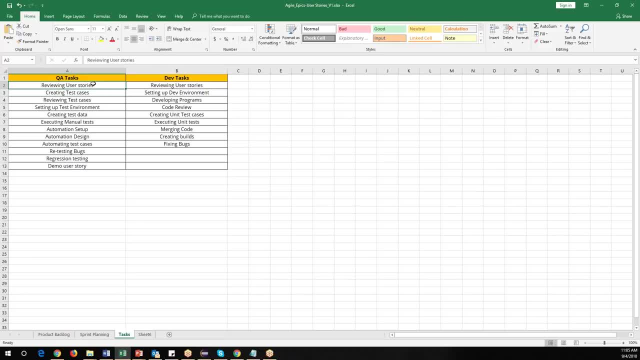 also create their own tasks, So normally QA task will be reviewed. user stories will be: creating test cases, reviewing test cases, setting up environment, creating test data, executing manual test cases, automation, test Automation, design automation test cases, retesting bugs, regression testing. demo to user story. 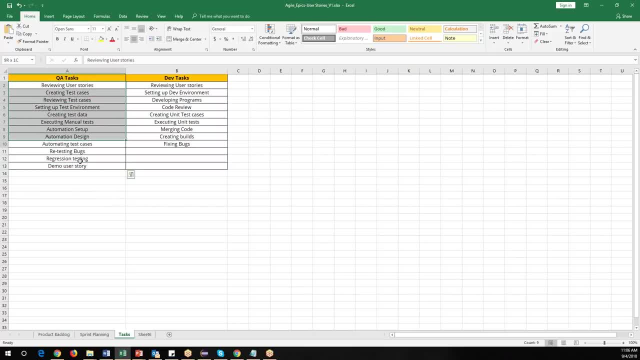 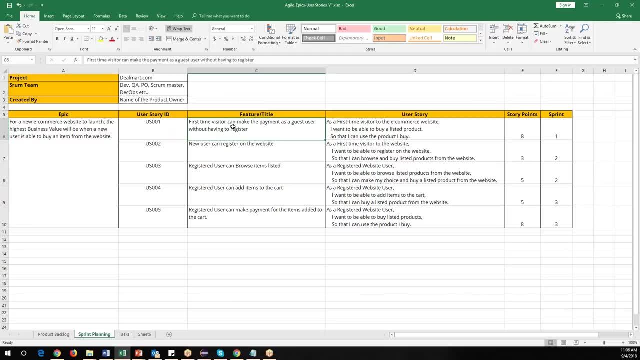 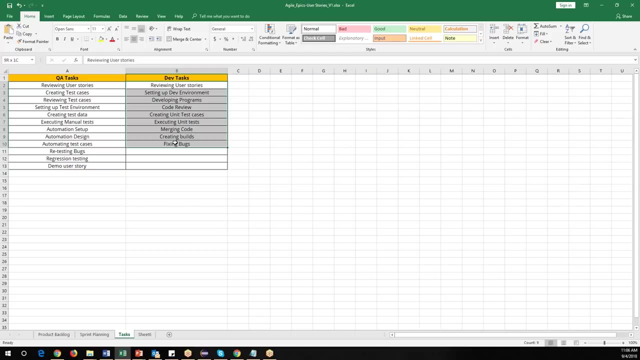 So all these are tasks for the QA. So once the QA is completed- all the actions, all the tasks for that particular story- then we will say: story is completed from the testing point of view and developer also should complete their own tasks for that particular story. and then we will say to the product owner: 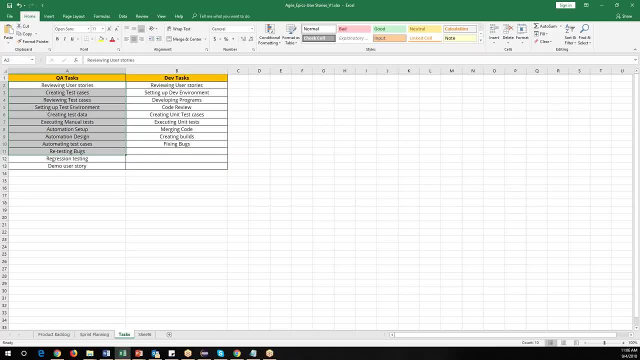 Okay, this story is completed. all the QA tasks have been completed, all the dev tasks have been completed. Okay, And then we will say to the product owner: okay, story is completed, So this is ready for demo. and once the demo is done, then product and user approved that. 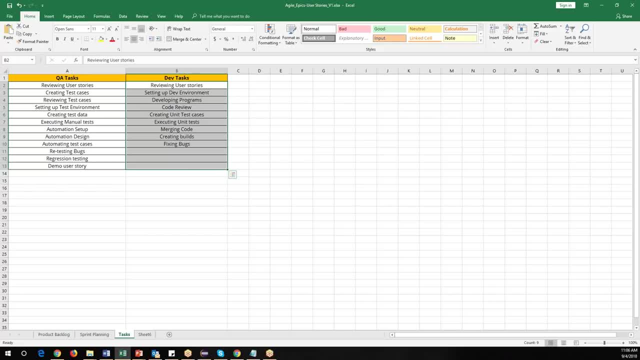 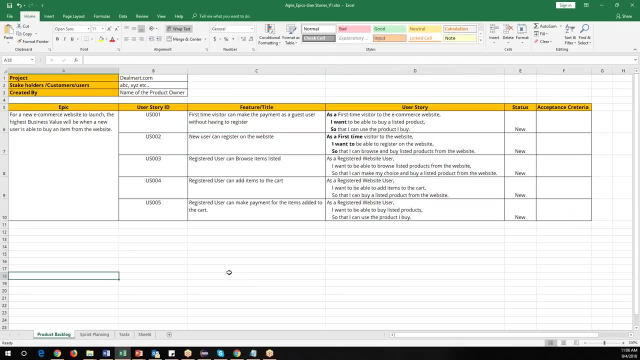 particular demo, then the story will be closed. Okay, then we will pick up the other stories for the next sprint. So this is how the planning will happen. So this is how the agile process will work. Okay, Now, in the next session, I will tell you how we can do all these activities. 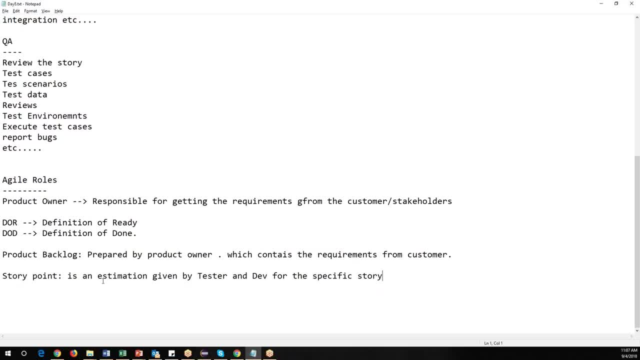 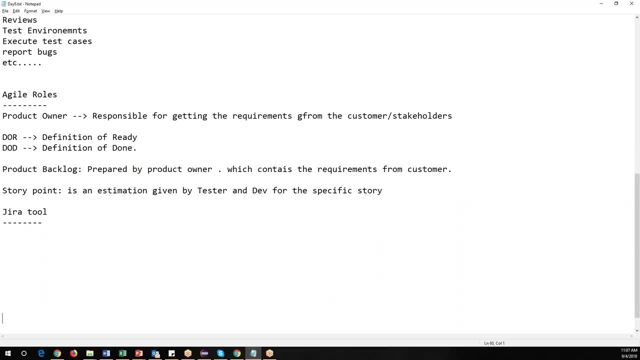 By using Jira tool. So Jira is basically used for multiple purpose. So Jira is a very popular tool currently in the market. So by using Jira we can perform a lot of activities. We can just so manage agile process, the complete agile process. 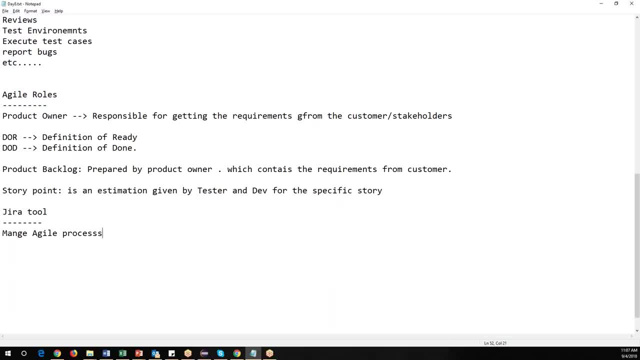 We can manage because agile process management in the sense we can create a backlog, We can create spin to stories, We can create the sprint, We can plan, We can use for that particular Sprint, We can update the statuses, We can create the task. 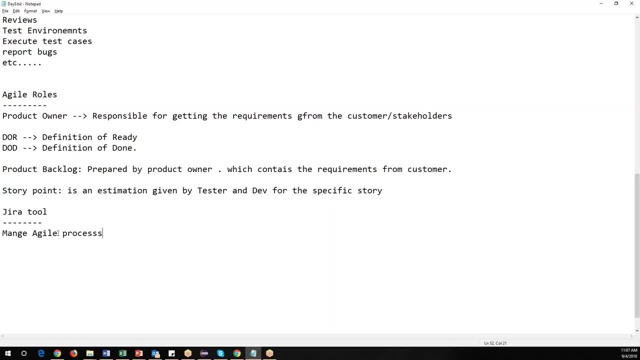 We can update the task. So all these things, whatever so far we discussed everything we can do by using Jira tools. that is called as a managing agile process. managing agile process, and not only this: by using Jira tool, We can also write our test cases. 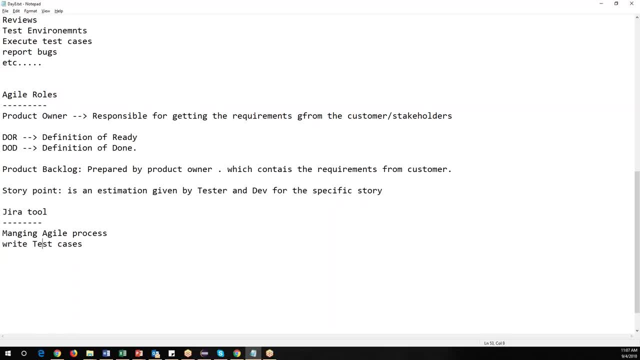 We can also write our test cases in Jira tool and also we can execute our test cases. execute test cases. execute test cases and we can update the status Of test cases, whether it is passed or failed. update the status of test cases. So managing agile process in the sense we can create backlogs and we can create Sprints. 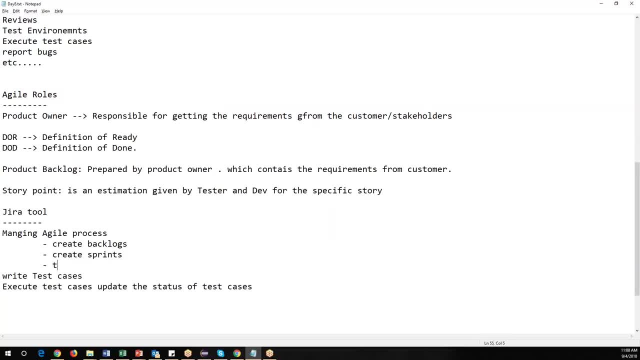 Okay, so we can create Sprints and we can create tasks and we can update the story status: story status in scrum board. story status in scrum board. So all these things we can do by using Jira tools, So we can create back logs.